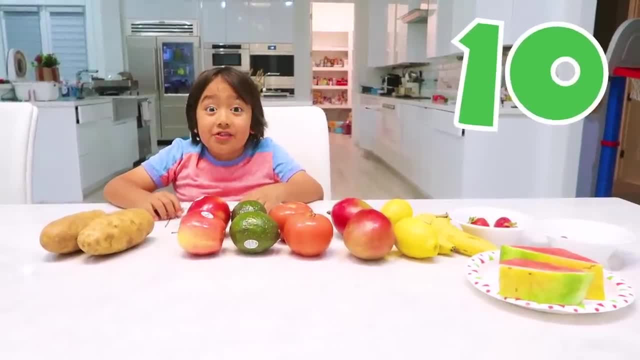 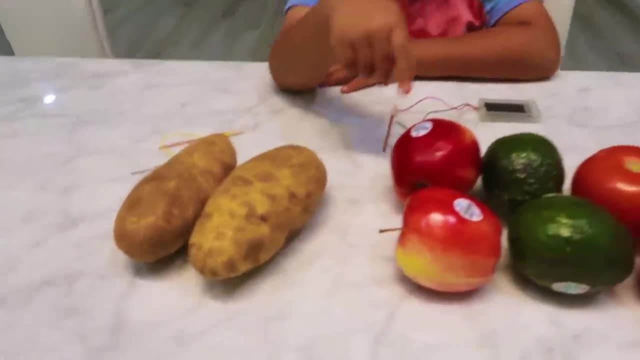 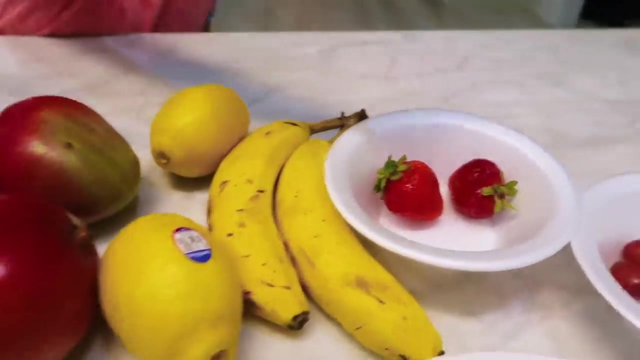 Hi guys. so today we're going to be using 10 different vegetables or fruits and we're going to see if they can power this alarm clock. So we have potatoes, apples, avocados, tomatoes, mangoes, lemons, bananas, strawberries, grapes and watermelons. 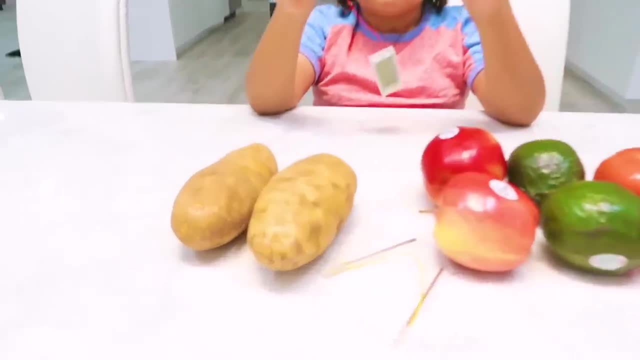 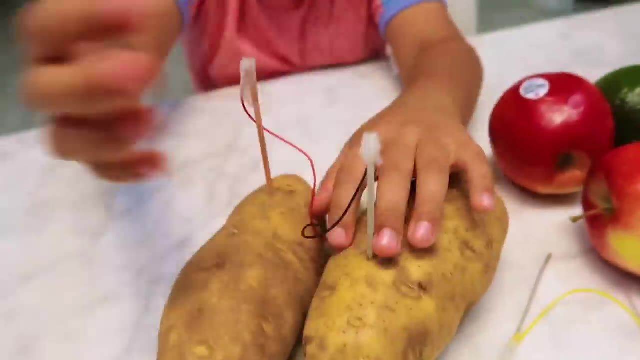 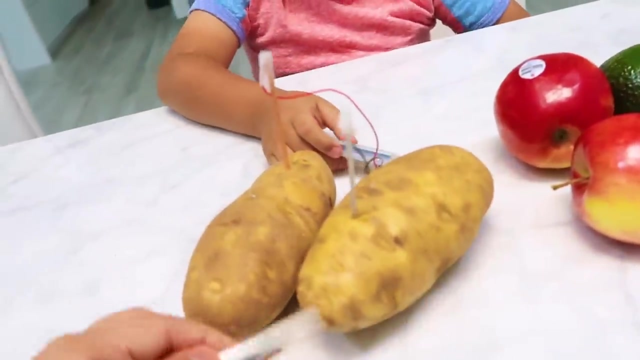 First we're going to try the classic potato. It was made for potatoes, so I think it's going to work. Three, two, one. So, if you notice here, look at the alarm clock. Is it working yet? Not yet. We got this kit online, so it comes with a magnesium wire and a copper wire. 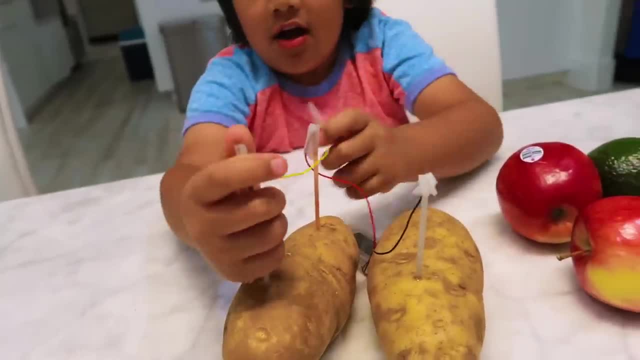 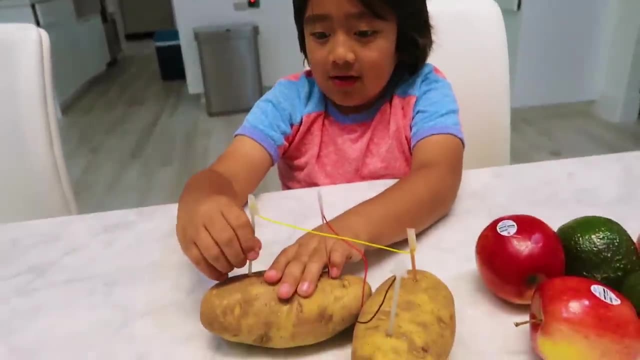 You have to connect this two, This Uh-huh, Hi, Yeah, And here, All right, you tell me, is the alarm clock working? Look it's working. Yeah, it turns on. It's got enough energy. 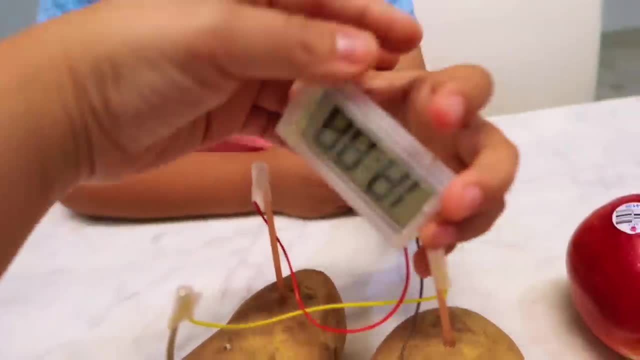 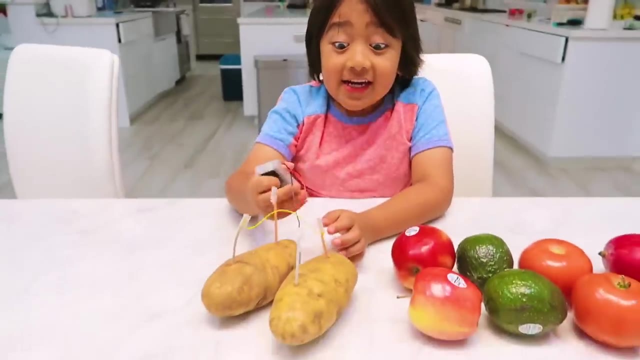 Yeah, so we have to manually set it. but you know, there it is, A potato works. I'm going to use a potato for my alarm clock tonight. Okay, now let's try the next one. Next, I'm going to test out the apple. 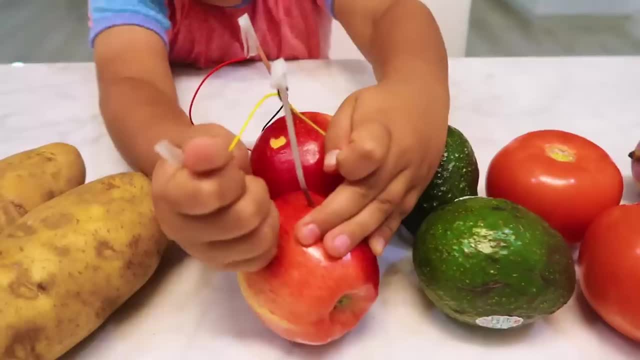 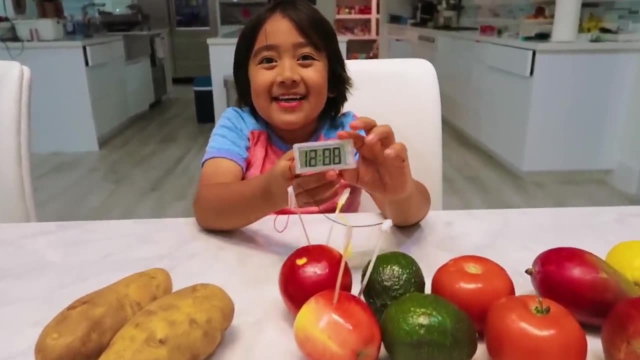 And do the opposite on the other one. Yes, like over here. There you go, Moment of truth. Does it work? It works, Yay, Okay, so an apple can also power. You know it's true because look what happened when I take out one. 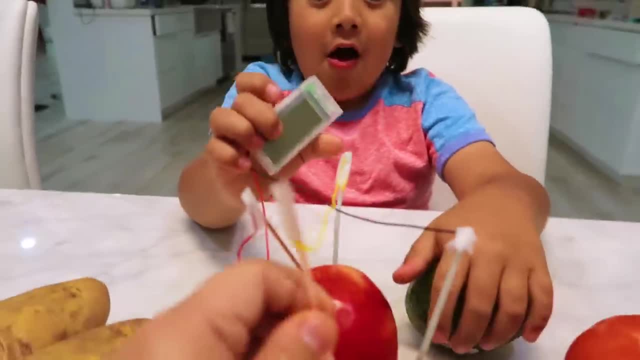 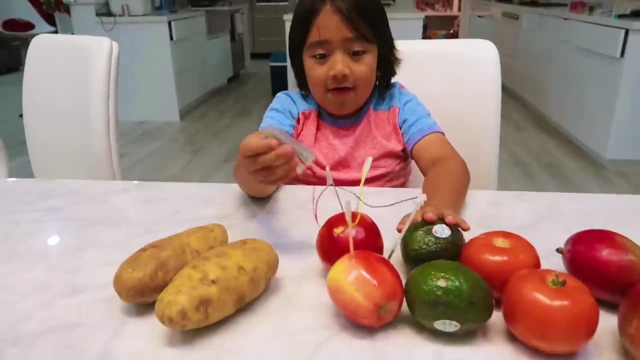 Okay, if I take out one, it stopped working, But if I plug it back in it works. I'm really interested for this one, The avocado. Yeah, Guys, let us know if you think avocado can power on the alarm clock. 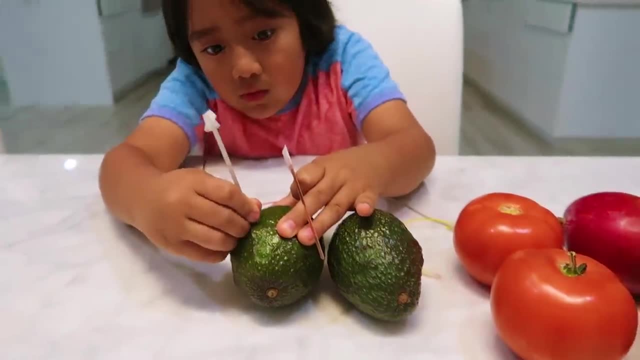 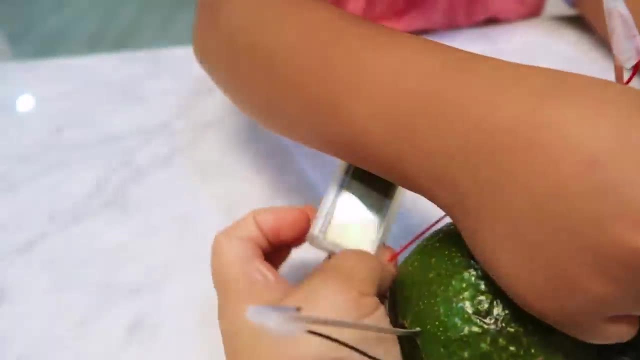 Now we're going to try the avocado. Ooh, ooh, ooh, ooh, ooh, Will it? Oh, I think it's going to work. You think so. Yeah, You guys notice, right now nothing's on right. 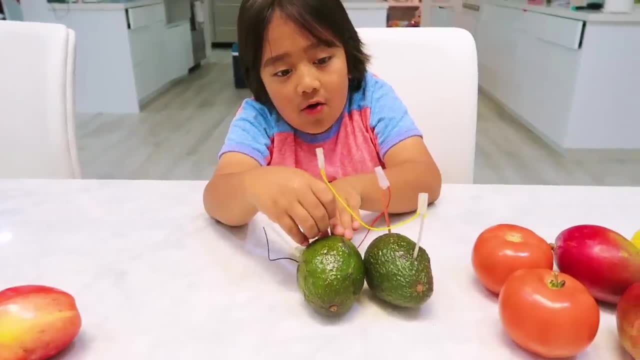 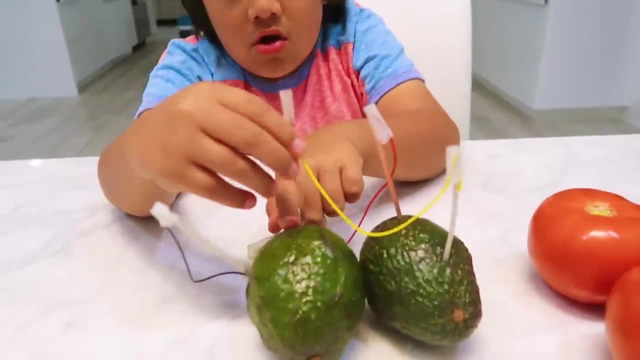 So it doesn't work right now. So Ryan's going to put it in. Can you use an avocado alarm clock tonight? Wait what I saw. I know What I'm supposed to put this. No, that's right. 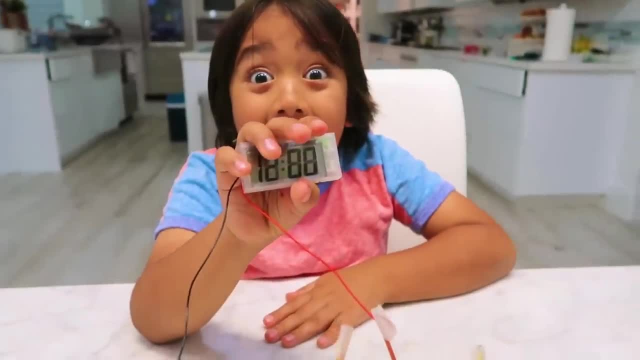 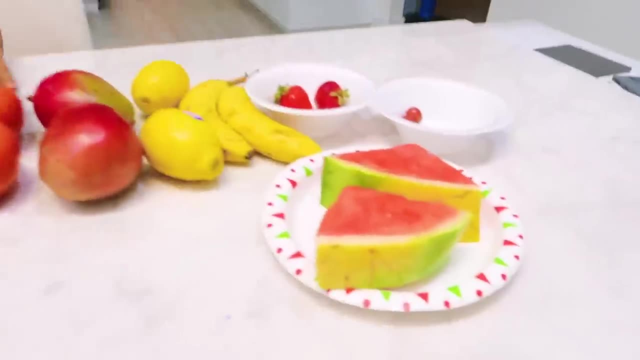 Yeah, it's supposed to be opposite. Uh-huh, You need that to complete a circuit. Does it work? Avocado work, Whoa? Now, the most interesting one is one That's true, That one we're not sure. 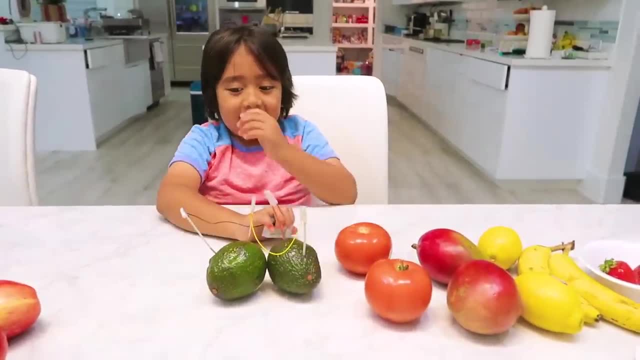 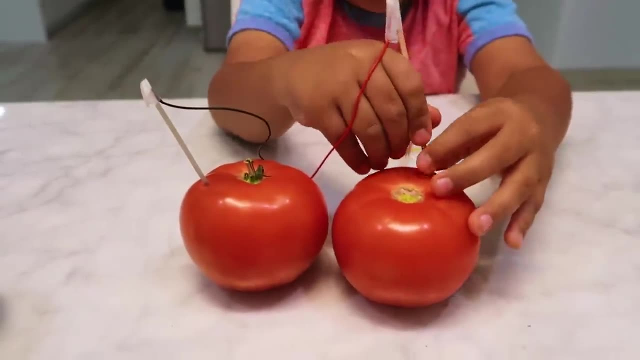 Also tomato. Wait, no, I think tomato will work, Tomato will work. Okay, let's see. Now we're going to try tomatoes. They're really messy, Don't poke it too hard. There you go, Pop And like this: 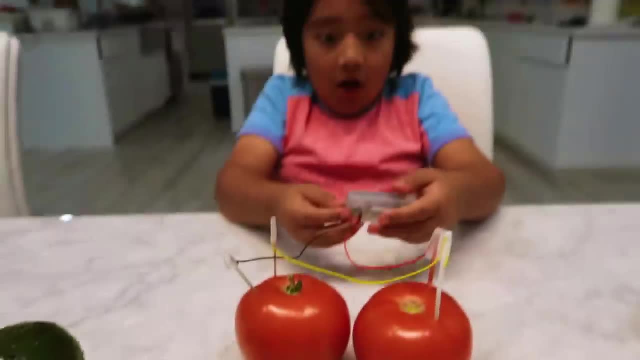 Does it work? It works, It does work. Wow, Maybe we do need just fruits and vegetables Power alarm clocks. You think fruits and vegetables can power on your iPad? Oh, That's a fun experiment to do later. Ooh. 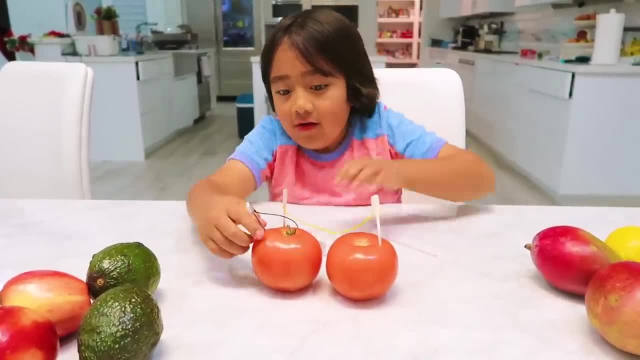 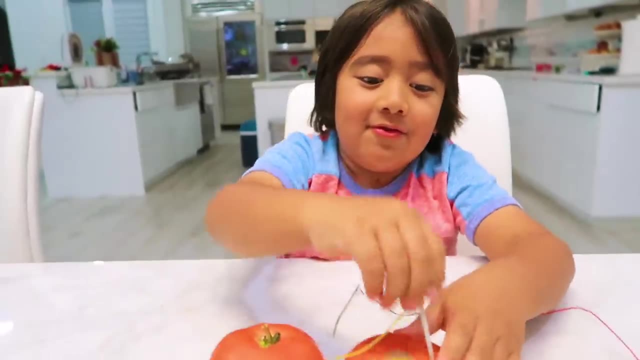 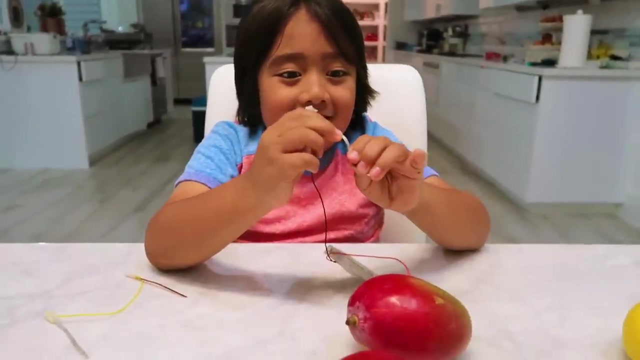 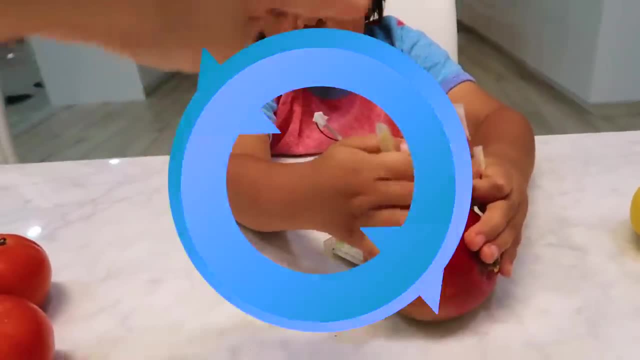 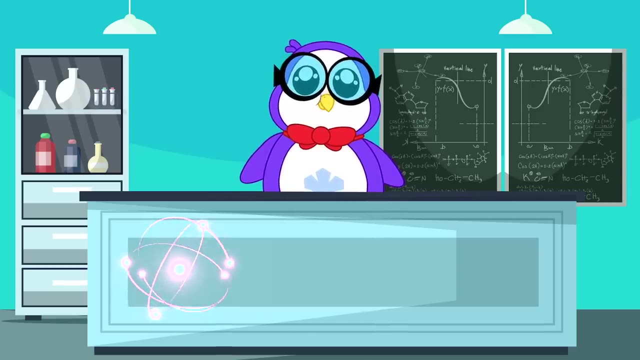 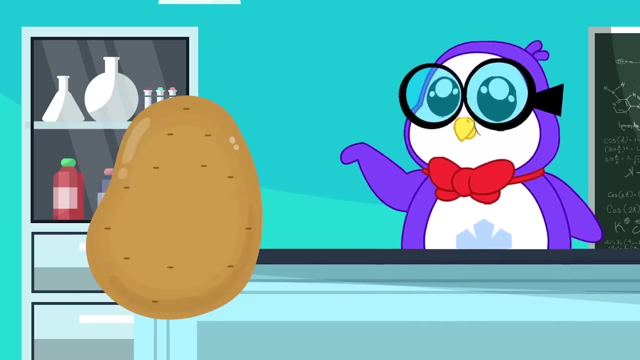 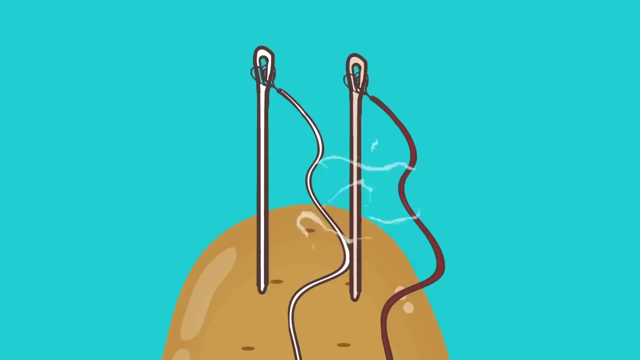 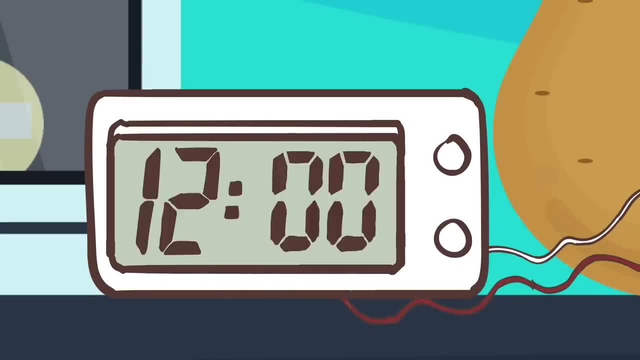 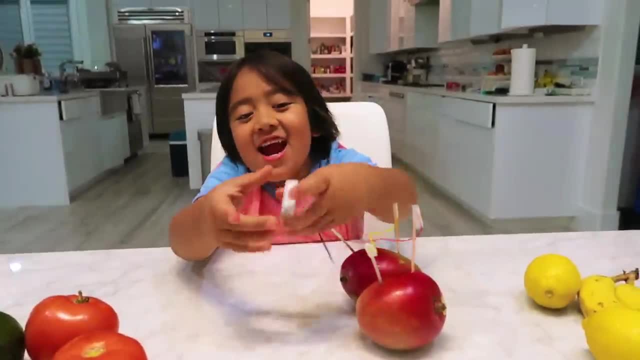 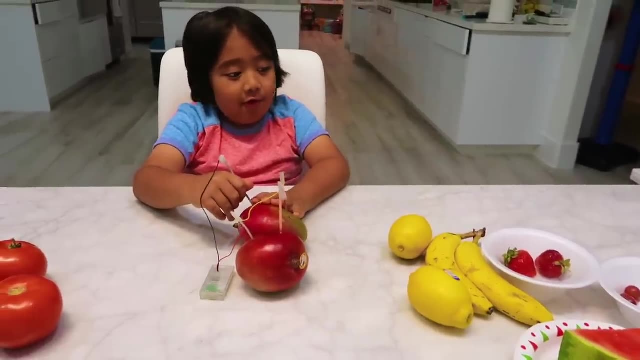 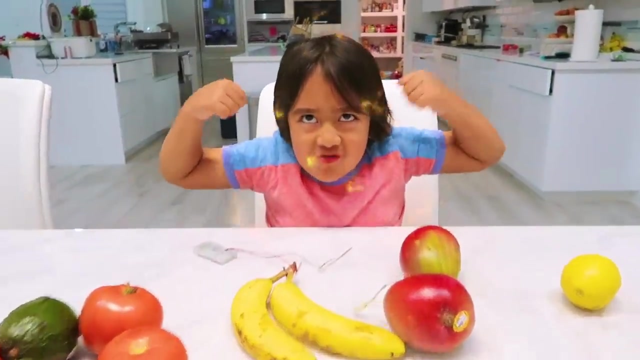 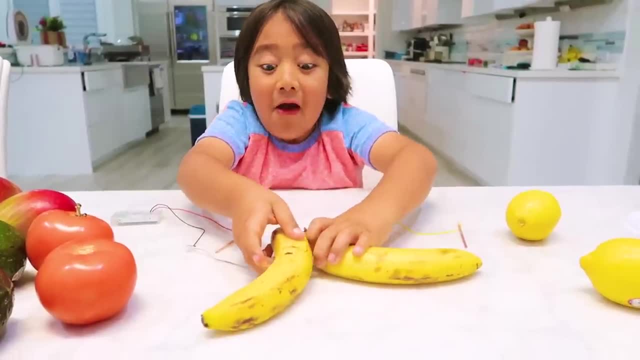 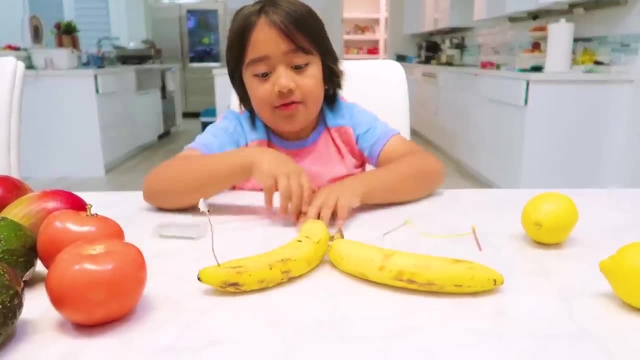 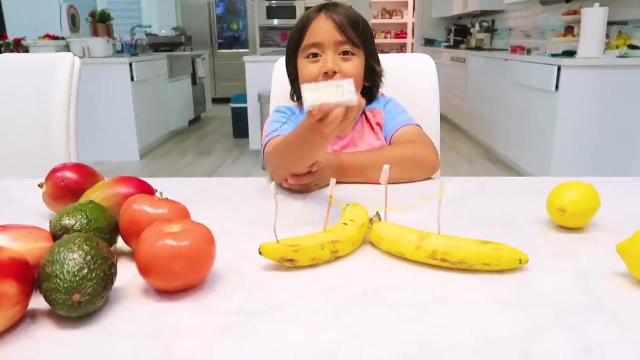 Okay, Now let's try banana. I'll try it like this. Okay, So it's easier to do positives and negatives. Well, I'll put it here. Yeah, put it anywhere you like. Well, Enjoying a different time, but yeah. 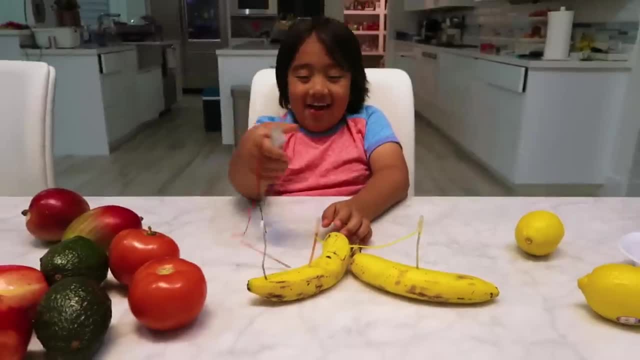 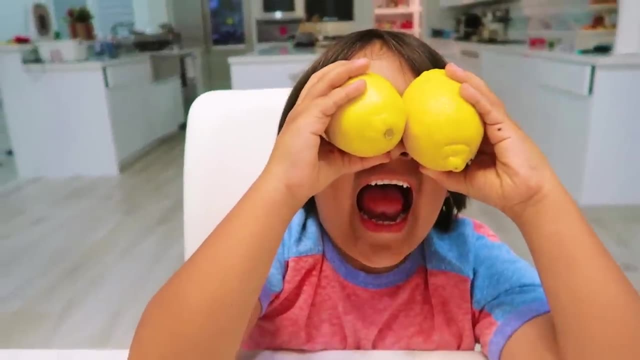 Oh, it does work. yay, You can have a banana clock. Oh woo-hoo. Now let's try banana whoa. What do you think, Ryan? The lemon's gonna work? Yeah, I think so. Oh yeah, it's gonna work if it's hard to poke in. 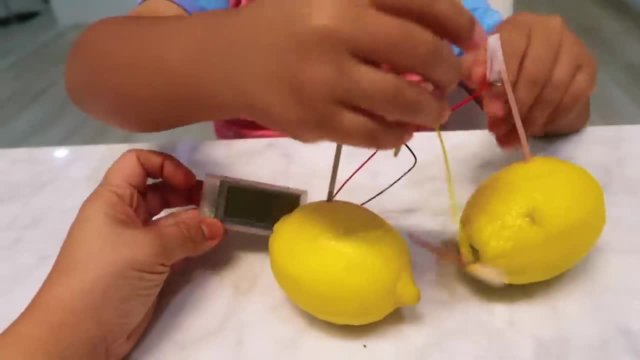 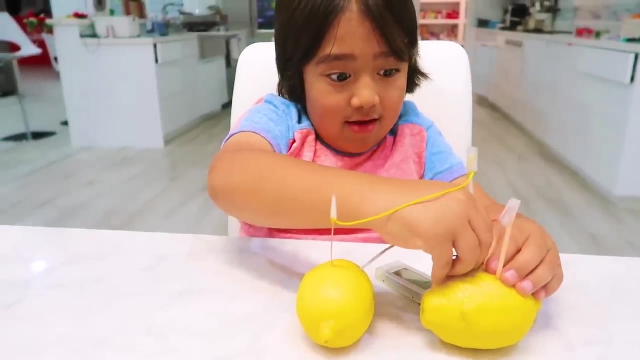 See, it has a smell. See, right now it is not on you guys. Three, two, one. What do you think it's gonna do? work or not? Definitely work. I don't even have to poke it in. 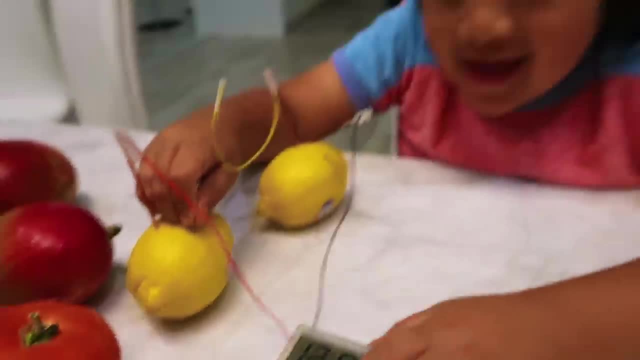 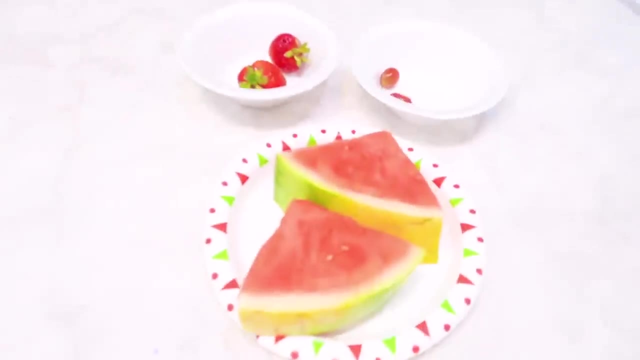 What. That's crazy. So I guess you don't really need a lot of power. So so far everything works, so far. Oh, Which one do you want to try next? These three I'm very interested in? Yeah, I'm gonna try this one. 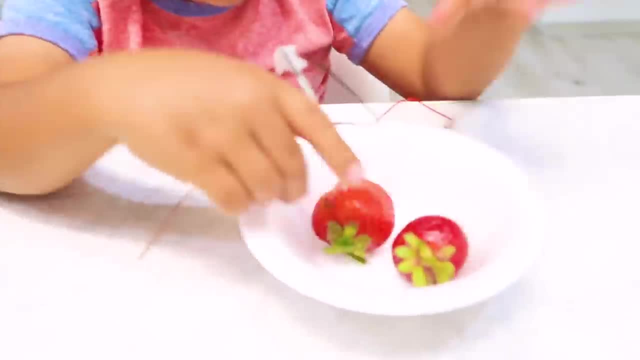 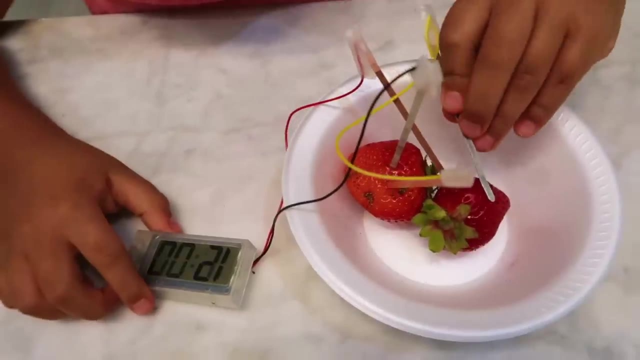 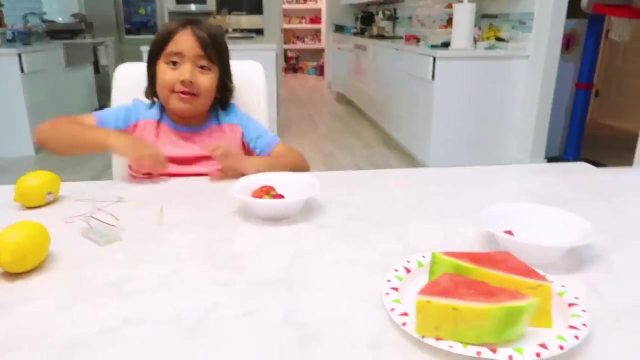 The strawberry. Strawberry, You barely have to poke this in. to poke it in, I wanna see if we can do the same thing we did with the lemon. Oh, good idea, Look we got it. Wow, very cool. Which one do you want to do on here? 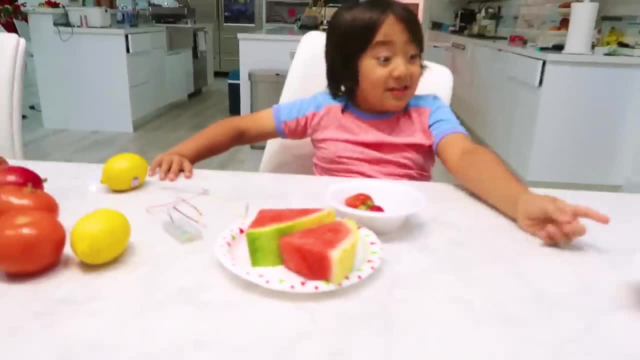 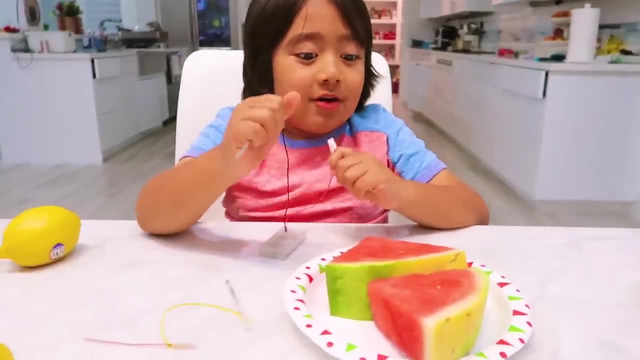 grapes or watermelon. The watermelon- Okay, because grapes it's so small, I know. Is it gonna work Because it's so tiny? You think watermelon's gonna work. Let's see, I think all of them are gonna work. 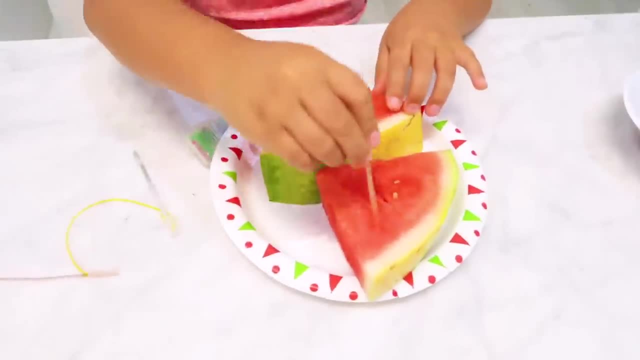 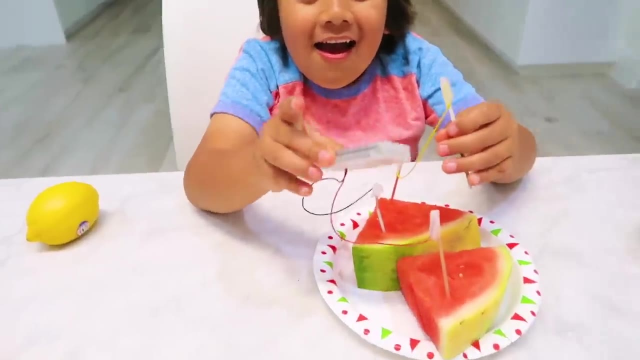 Oh, it's so easy to poke in. Yeah, What Is it working? What Guys? I didn't even need to complete the circuit, It just powers off with two. Wow, I didn't know watermelon's so powerful. 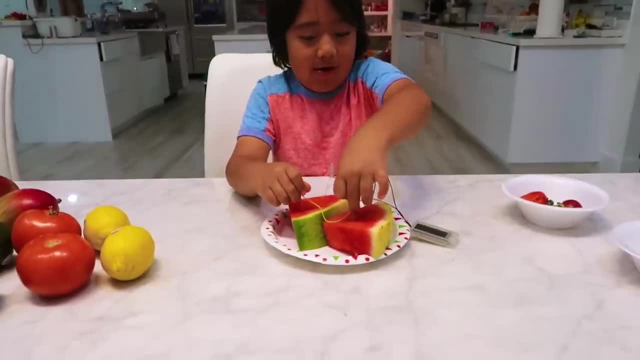 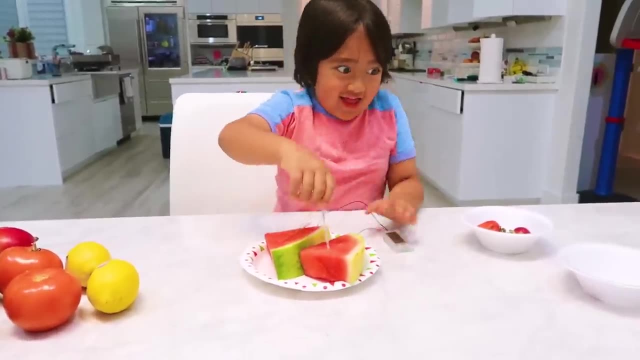 Well, I love it, But this makes it a lot more powerful. So it does work. yay, Really. Yeah, Let's try the last one in the most. Wait, how is this gonna work? I don't know, it's so small. 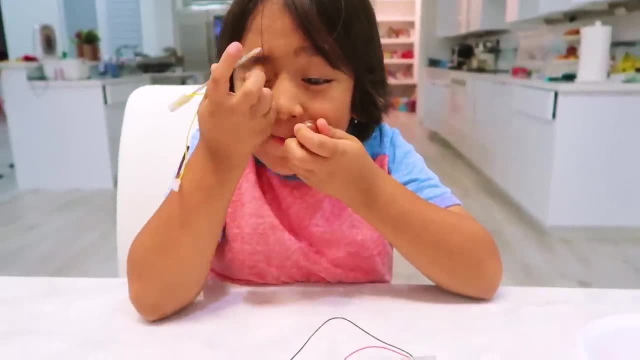 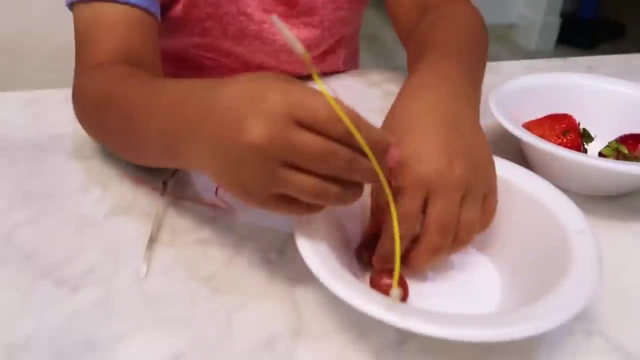 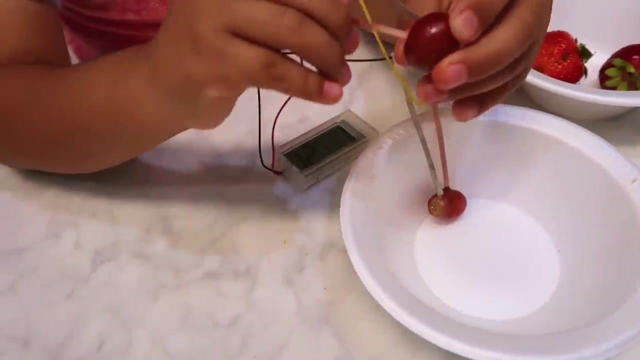 How are we gonna make it opposite and positive? You have to stick them very gently, Can you do it? Yeah, I did one, Now I do the other one And one here. So far it's not working. Let's see. 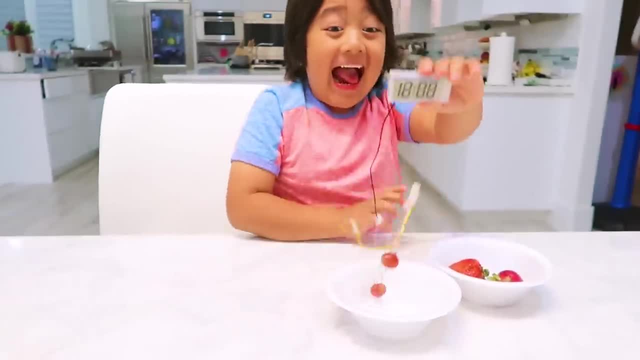 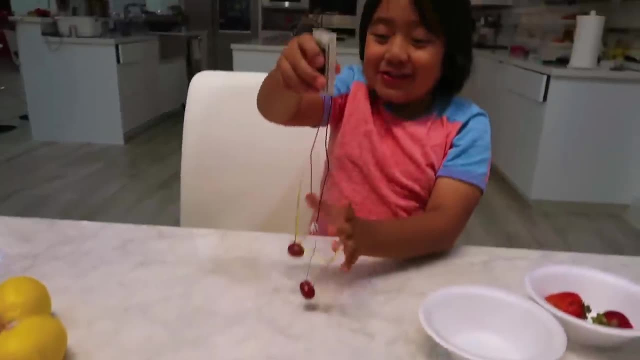 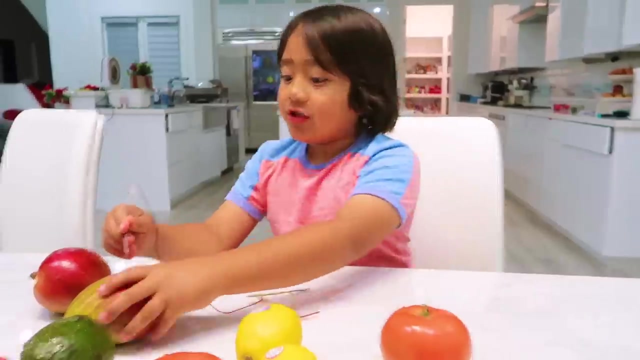 What It worked. Grapes can power on a clock. Look at that, you guys. Just two grapes, That's it. that's all we need Grapes. Don't need a whole potato, you just need two grapes. Well, what if you just try one of them? 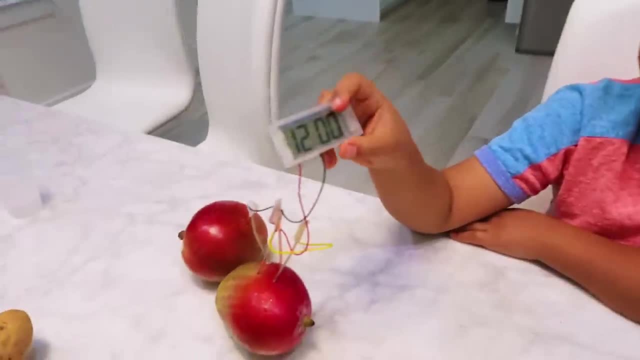 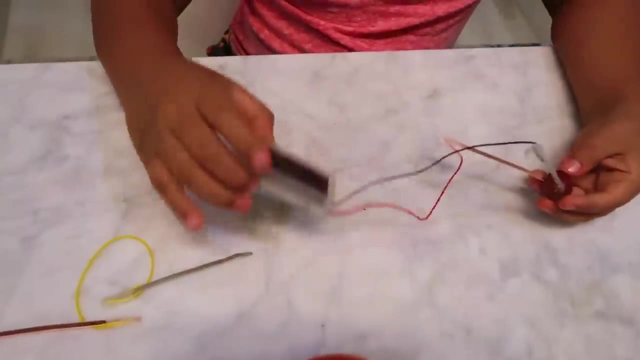 Yeah, With all of them, It's working. Yeah, all you need is one fruit, One grape. it is. It does work. look Just one, two. we don't even need to complete the circuit, It's so powerful. 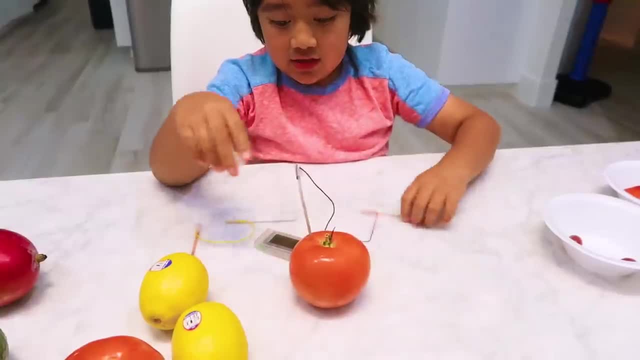 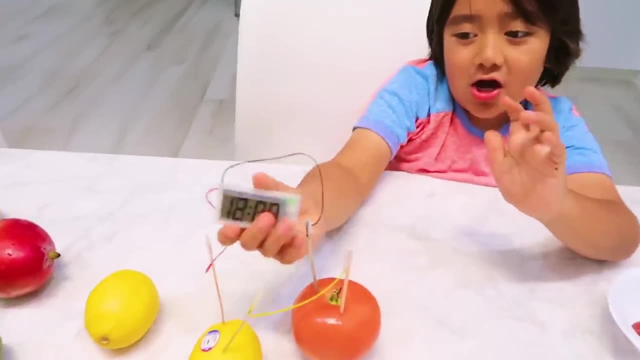 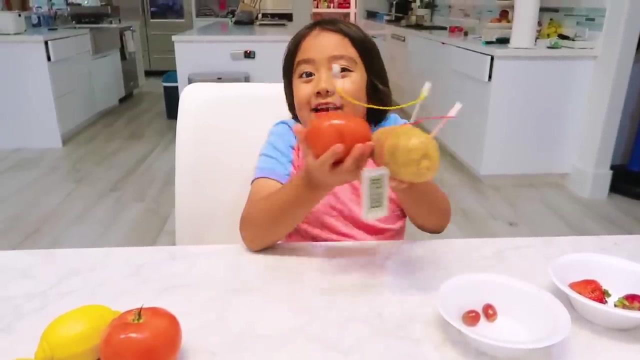 This is the most powerful. Yeah, I think all you need is one Ryan Like this. So Ryan's trying out different ones. So one tomato and one lemon, It works, Woo hoo. Okay, guys, I'm gonna take my alarm clock to bed. 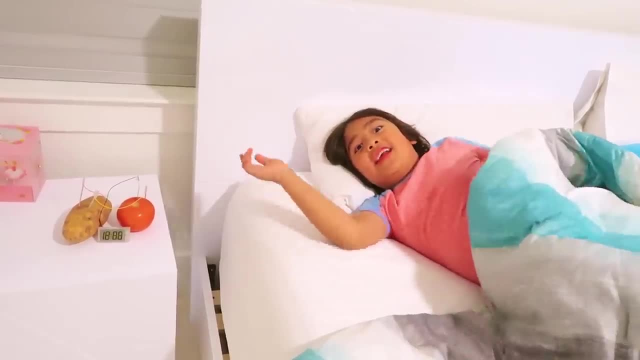 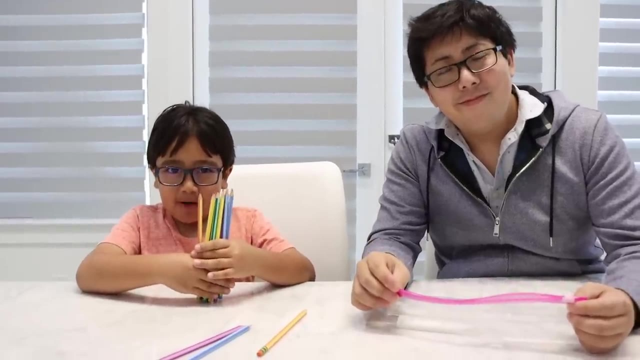 Let's go Bye, guys. I'm gonna go to bed now, And that's how you make a fruit and vegetable alarm clock. Hi guys, today we're gonna do a science experiment with pencils And we're gonna poke these pencils through a Ziploc bag. 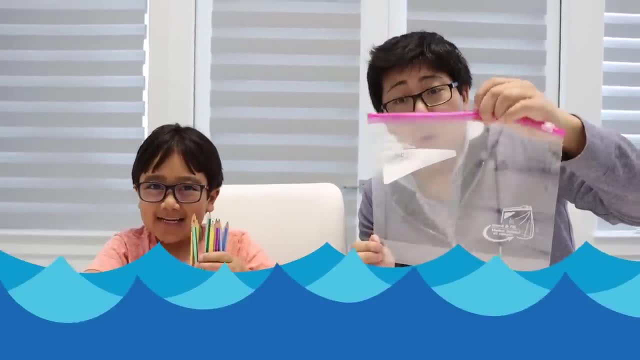 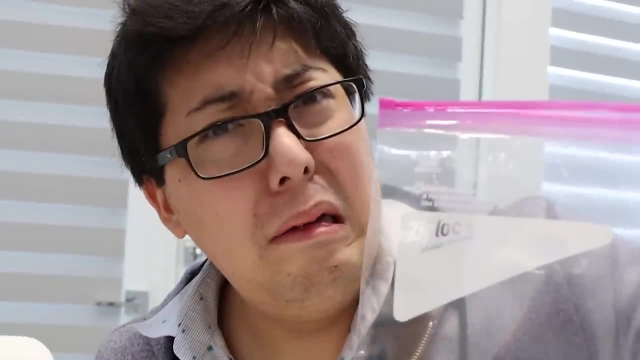 And the Ziploc bag will have water inside it. Whoa whoa, Ryan. so that means all the water's gonna leak through, Ryan, That's what you think, Uh-huh. First, let's put water inside the bag. 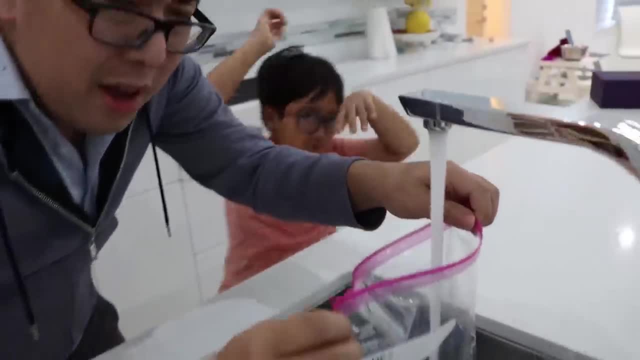 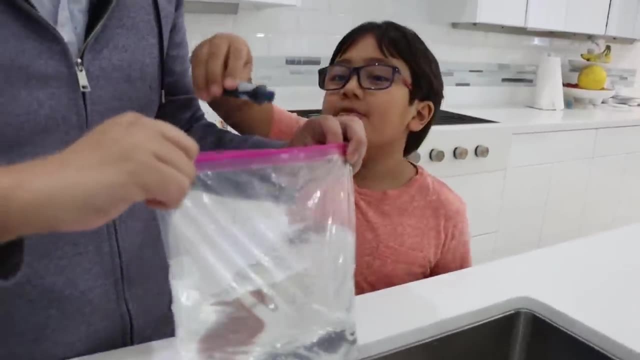 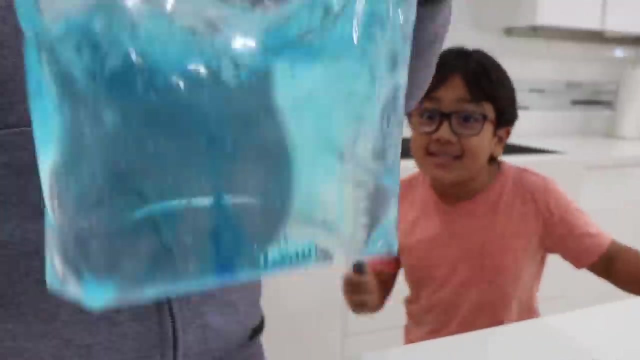 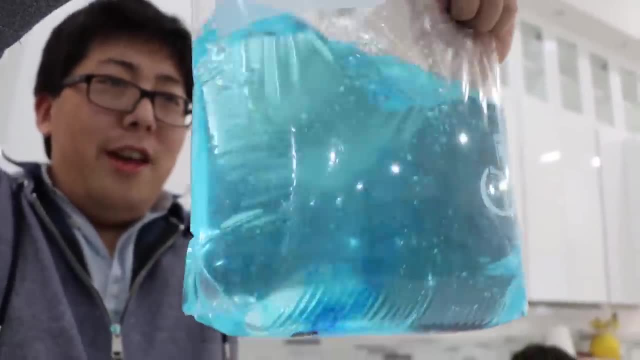 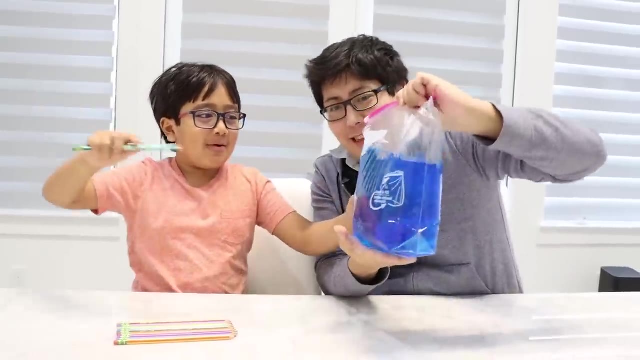 Look at the color Nice. look at the ocean Next up. we're gonna need a sharpened pencil. Don't forget to ask your grown up for help. All right, here we go. We're gonna poke it through Three, two, one. 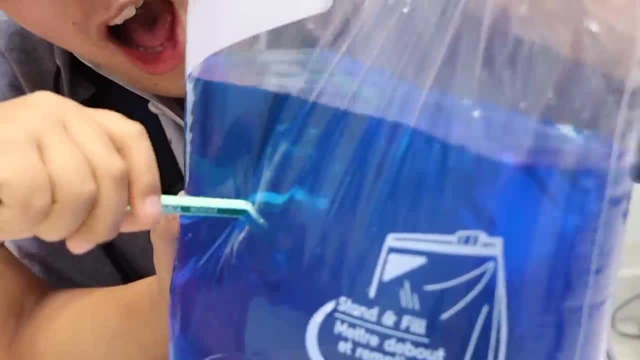 Is it gonna work? Yeah, it's not gonna make a mess, It's poking through. Whoa, look the pencil's inside. Oh, no way, guys, There's no water coming out. What? Why is it like this? 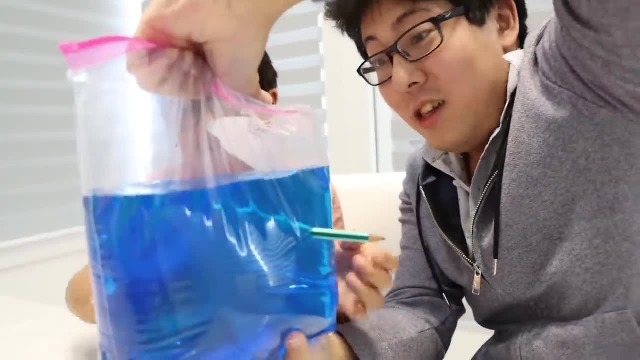 How's it working, Ryan? Whoa, Do more, Ryan. Okay, I'm gonna do a bunch of pencils. Whoa, What. What about you? try, Daddy. Oh, can I do it? All right, let's see. 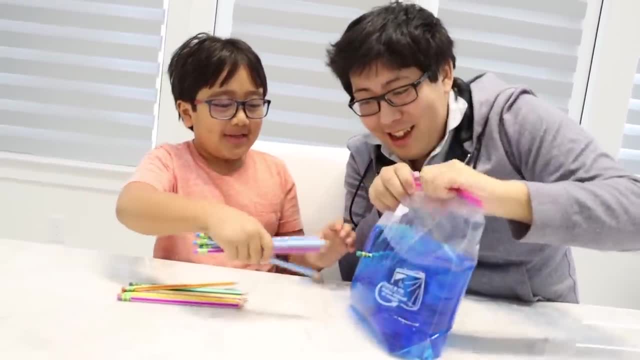 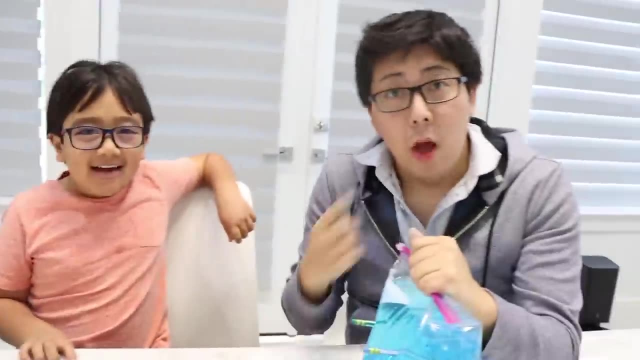 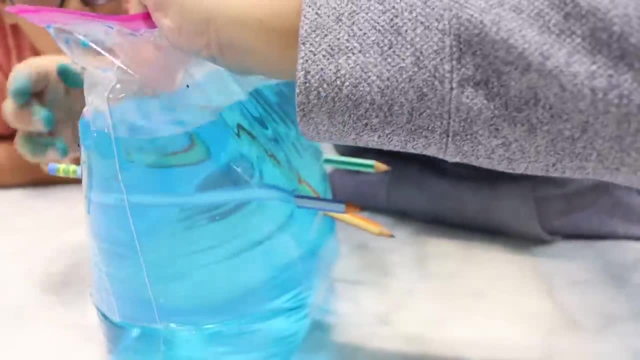 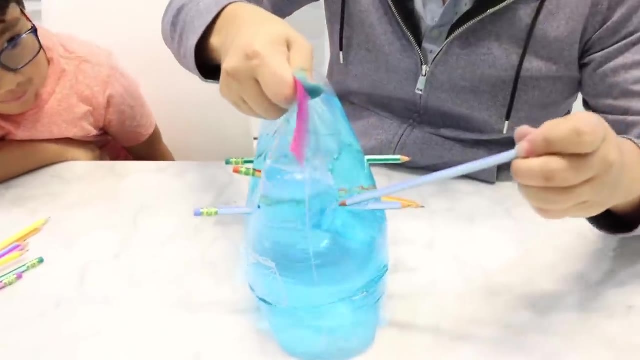 All right, All right, All right, Whoa It works. Whoa, That's cool. All right, let me do it from the opposite direction, Up Down. Whoa, Whoa It's working. Yeah, it is. 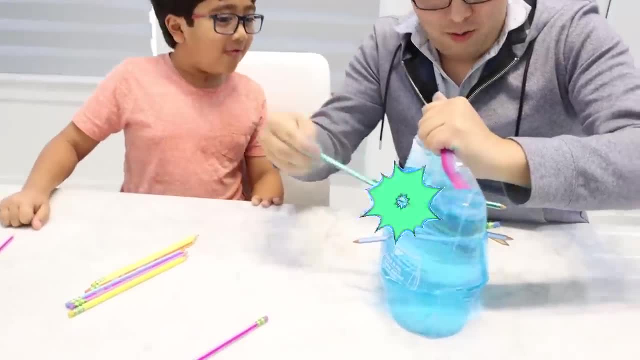 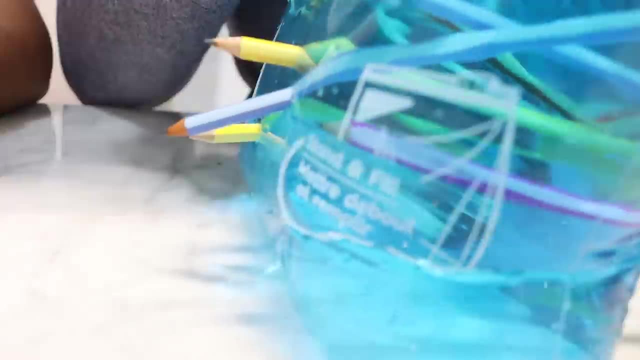 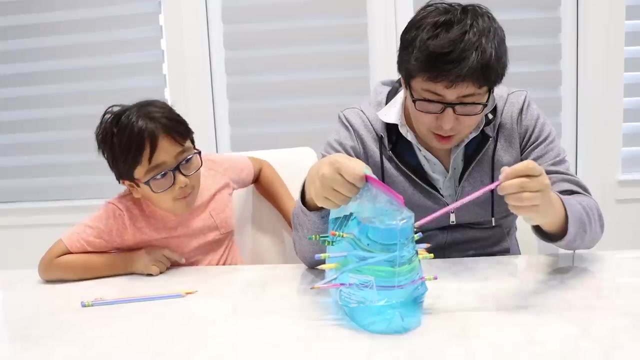 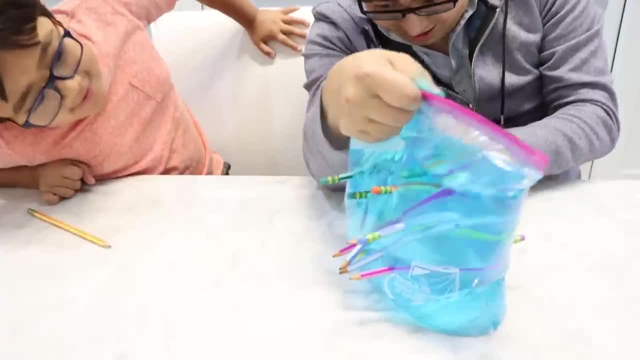 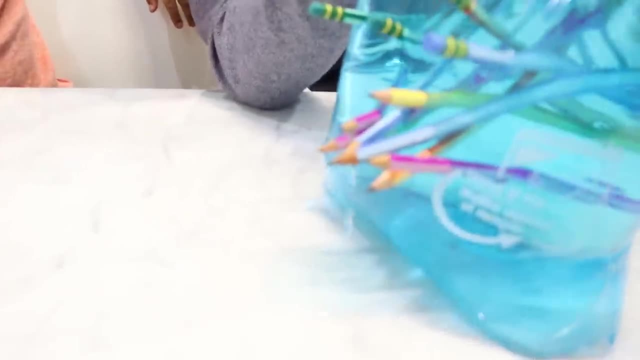 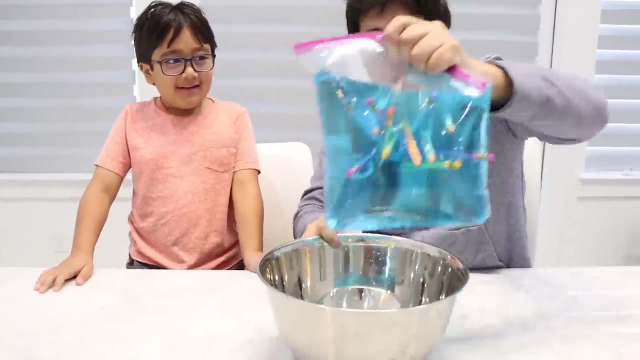 Let's see if I can do all of them. I think I poked too much, Daddy. what about we take out all the pencils and see what happens? Good idea, Just in case, let's put in the ball. All right, let's see what happens. 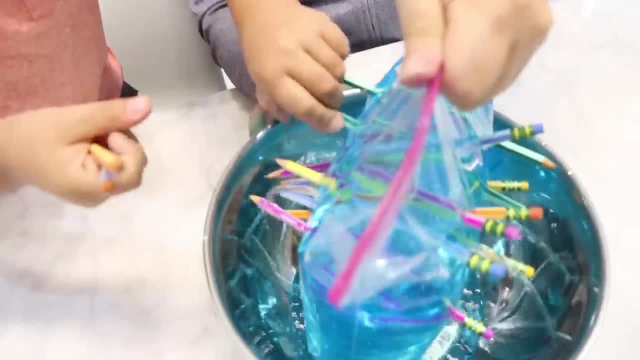 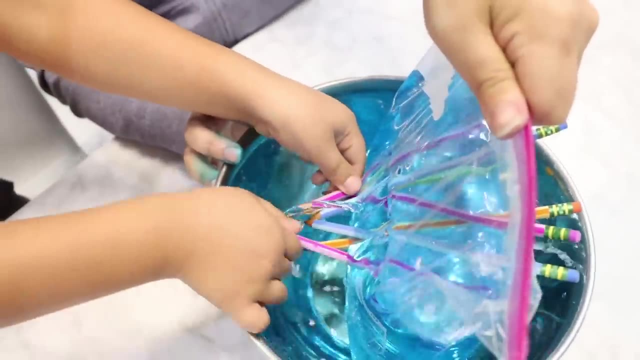 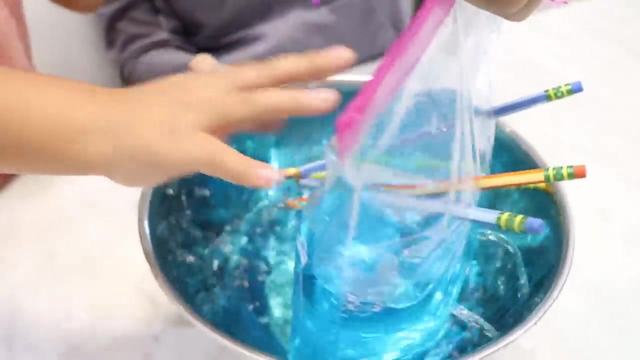 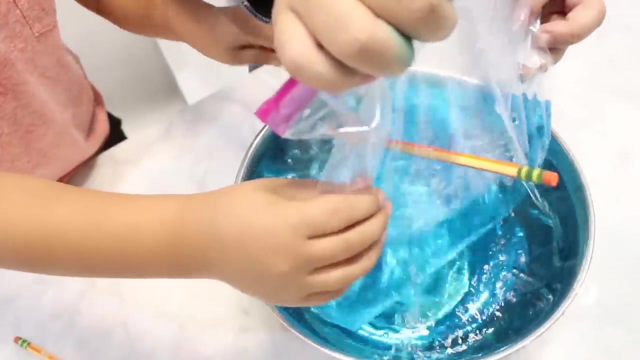 Oh, water's coming out. There's so much water, Water, Water, fall Water. those Whoa look at that. Well, there's so much water coming out. It's a shower, It's a shower, It's a waterfall of water. 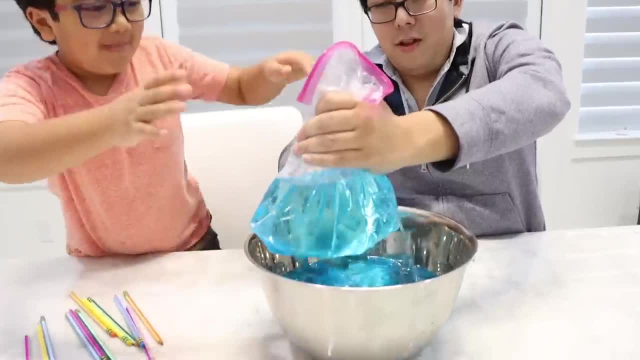 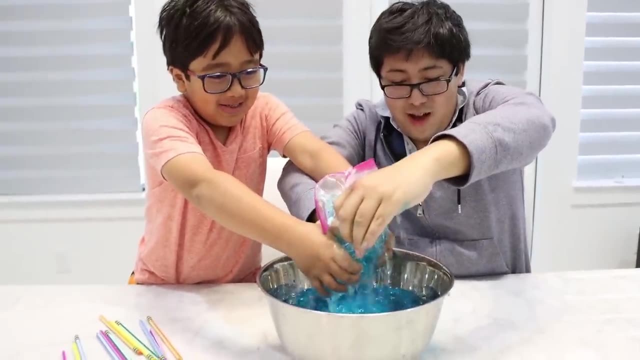 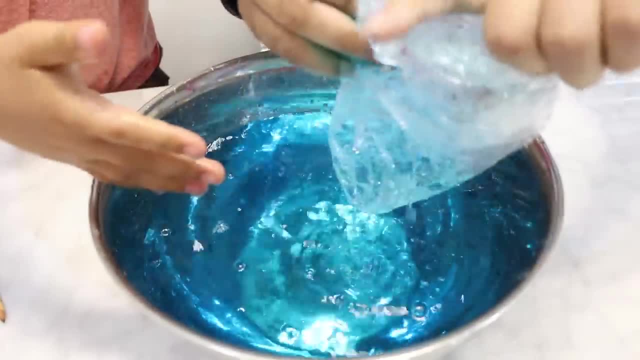 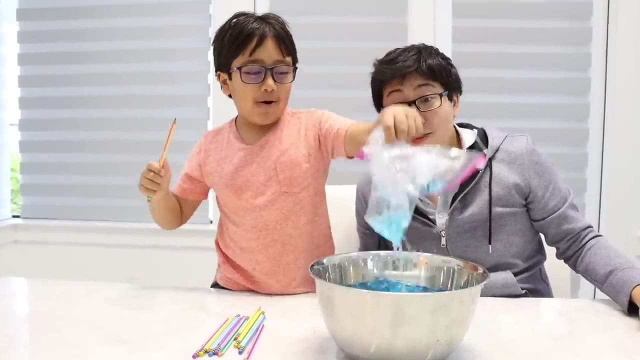 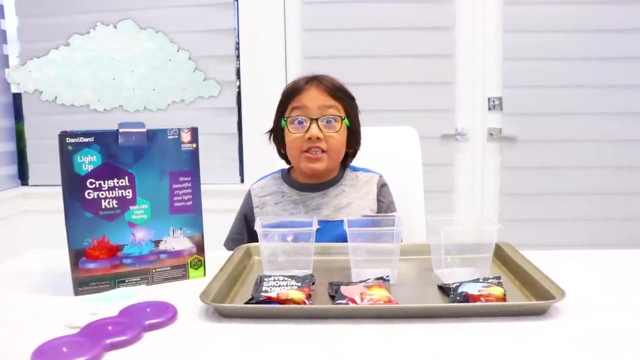 Whoa, Whoa, Whoa, Whoa. Big mess. Wow, It almost filled up the whole thing. Thank you for watching a science video about pencils poking into a bag. Did you know the most common crystals are salt and sugar. 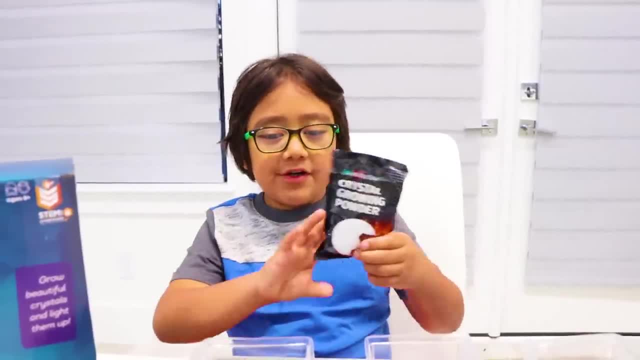 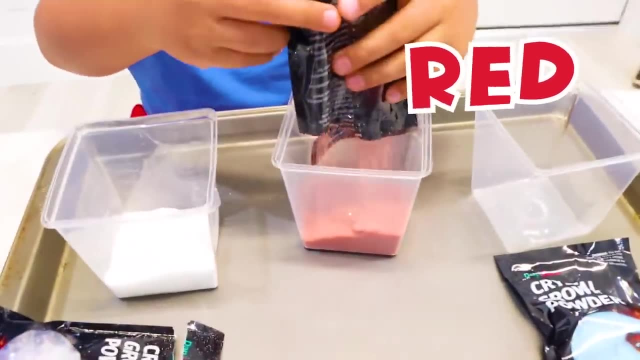 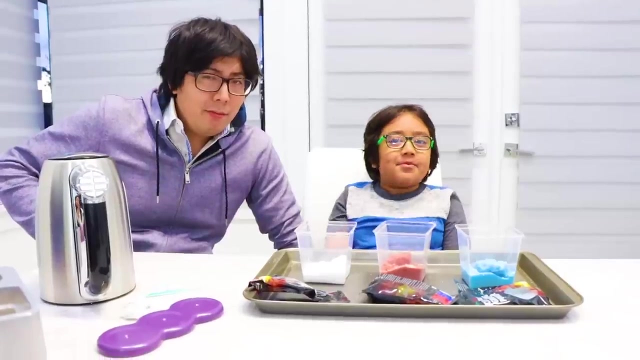 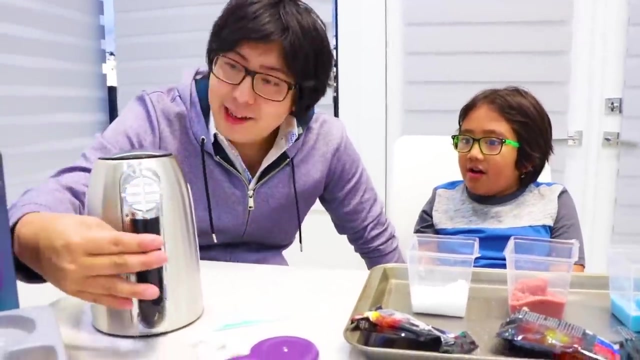 First up, The crystal powder. First we're going to do white, Next is red, Last is blue. Next up, you have to ask a parent for help. You have to put boiling water in. Yeah, you have to watch out because it's really hot. 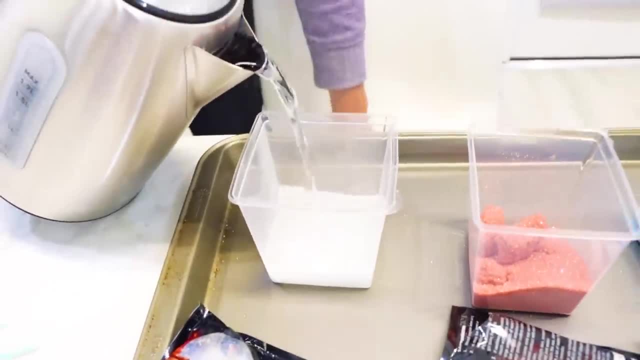 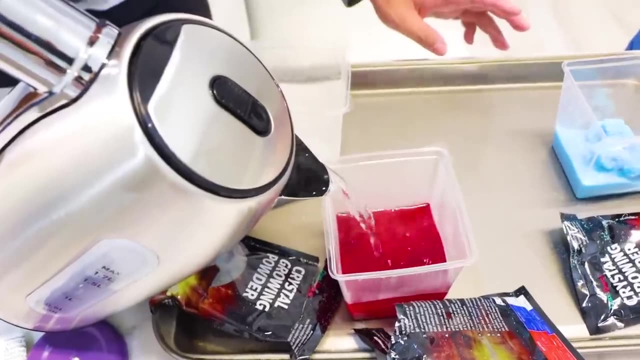 Whoa, You see the steam coming out. Be careful, I love the color. Look at it. Last one, Make sure you don't touch it. Thank you, Daddy, You're welcome Next up. be very careful, We have to store it for five minutes. 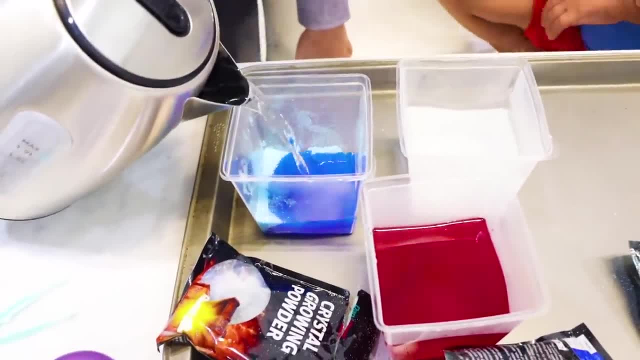 Okay, I think all the crystals are done. I'm going to put them in the bag. All right, Let's put them in the bag. All right, I'm going to put them in the bag, All right, All right, All right. 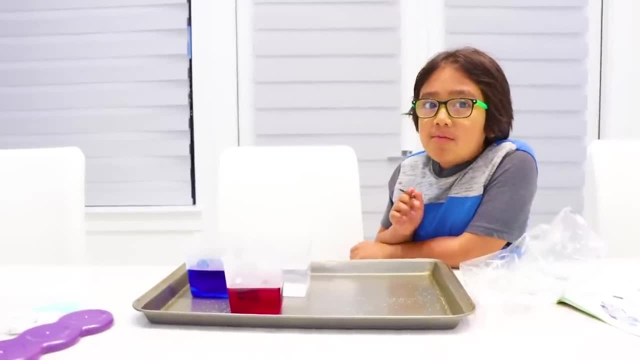 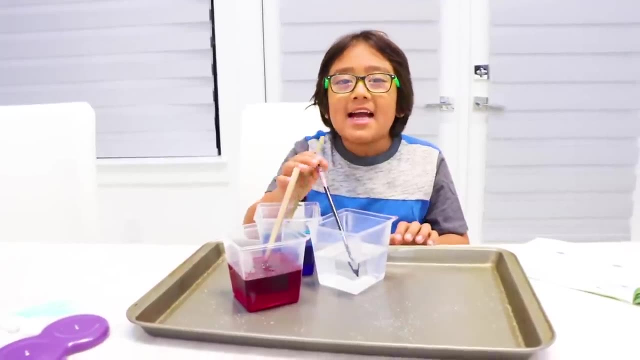 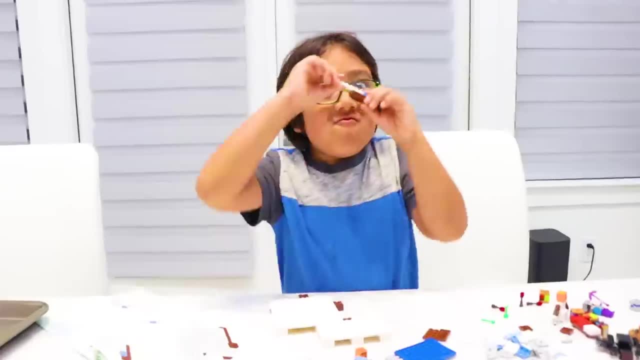 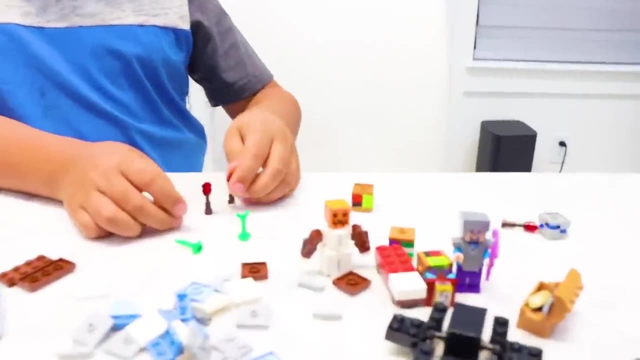 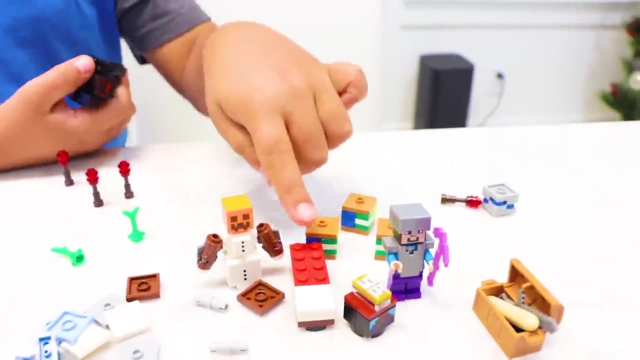 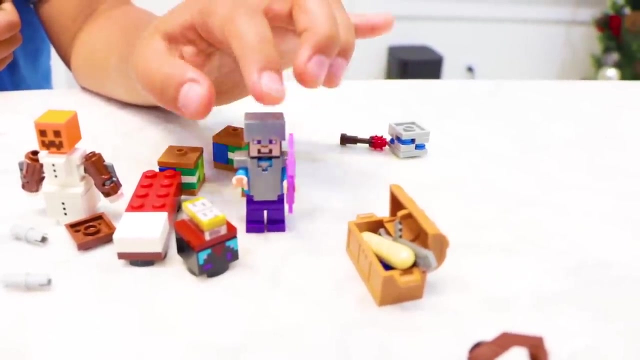 If you guys are curious, I'm building Minecraft. These are all the things I made so far. This is a snow golem, and these are bookshelves, and this is a bed, and this is an enchanting table, and this is Steve with obsidian pickaxe. 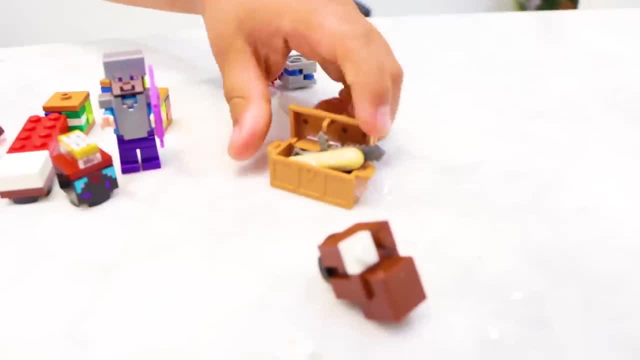 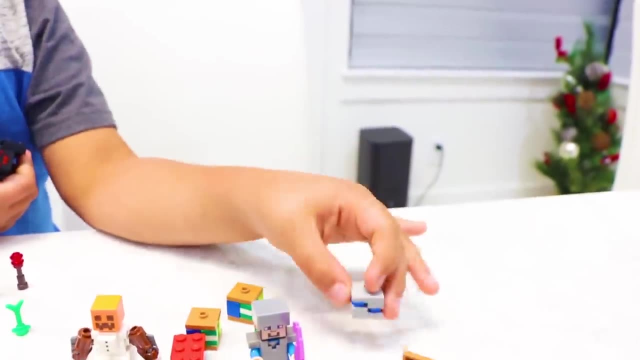 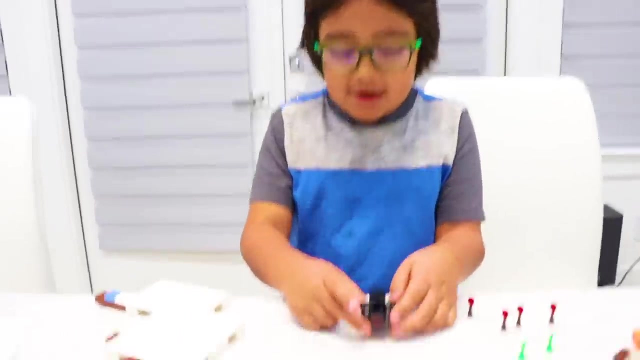 Me pickaxe, and this is a hidden treasure chest and this is a cow and this is probably an anvil. I don't really know what that is. and these four things are torches and I don't know what these are. And here's my favorite spider, Waddup. 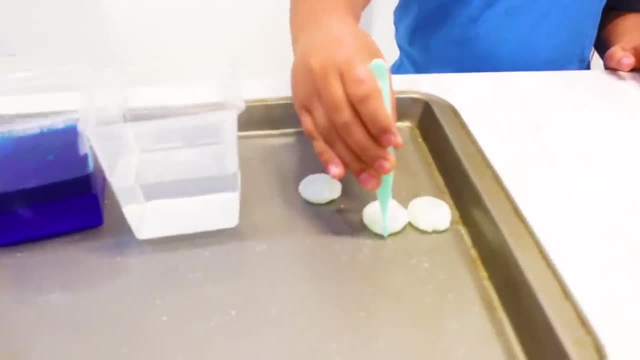 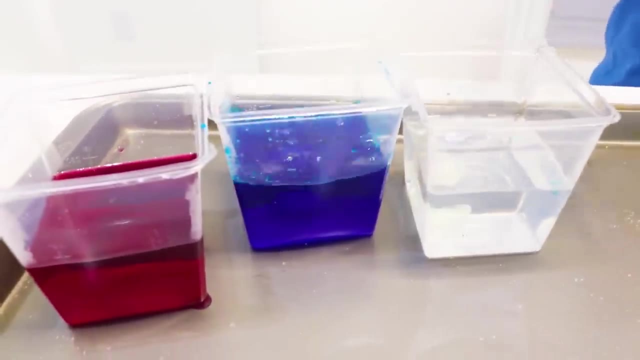 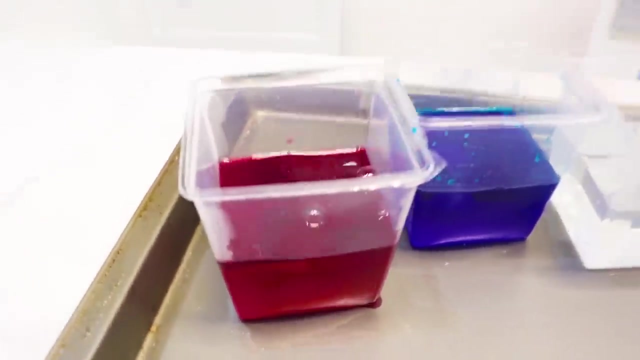 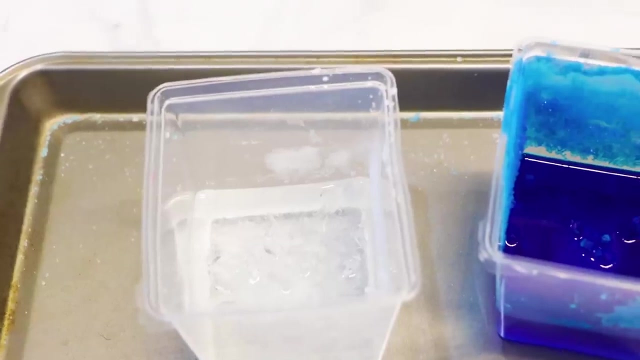 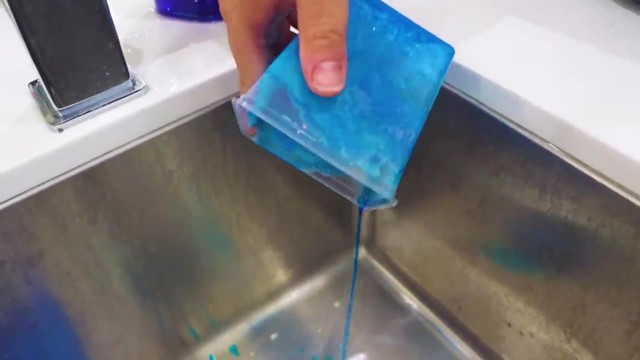 Now we gotta put in the crystal starters and we gotta put in the white crystals too. Now we just have to wait and see our crystal grow. Guys, it's been a whole week and look what happened. You can see the crystals inside white crystal now. 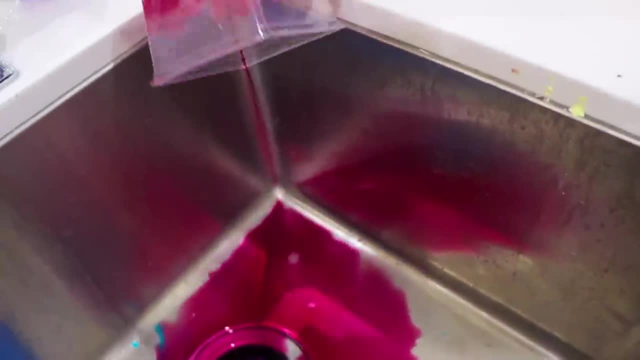 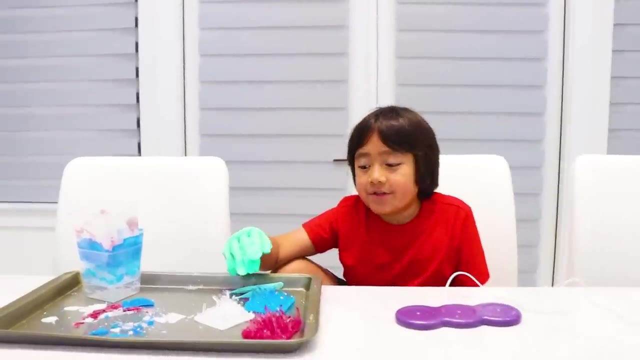 let's pull out the blue crystal. Now let's pull out the red crystal. Whoa, it looks so cool, But now I need to wrap this up. Now I need to wrap this up Now. it looks so cool. wait eight hours for it to dry. I took out the crystals. here's what it looks. 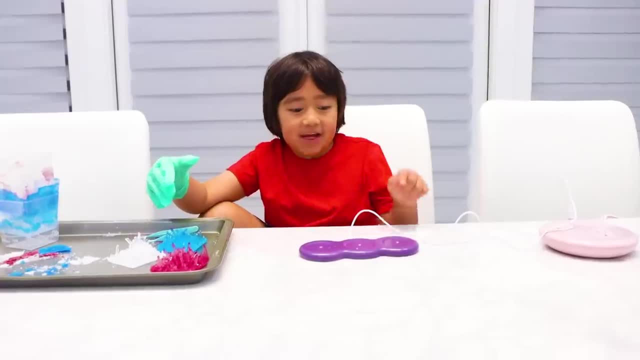 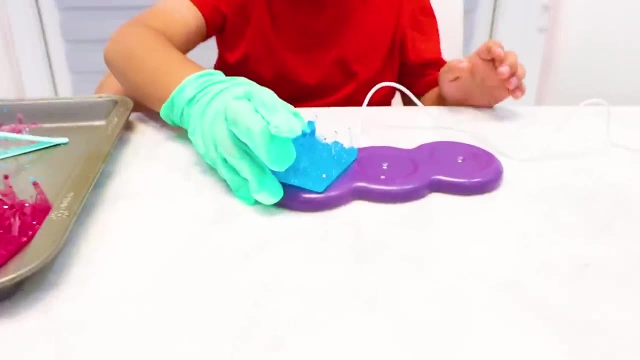 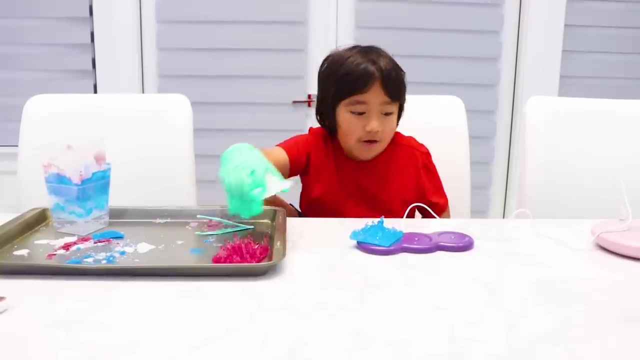 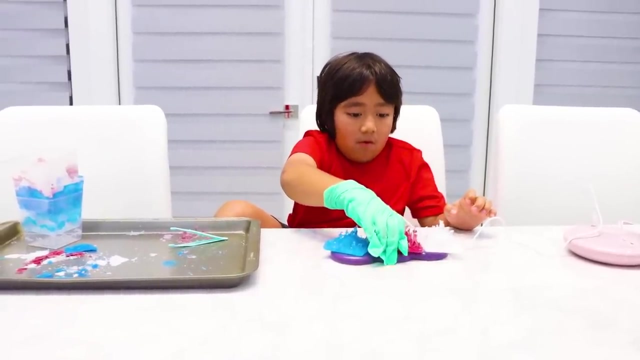 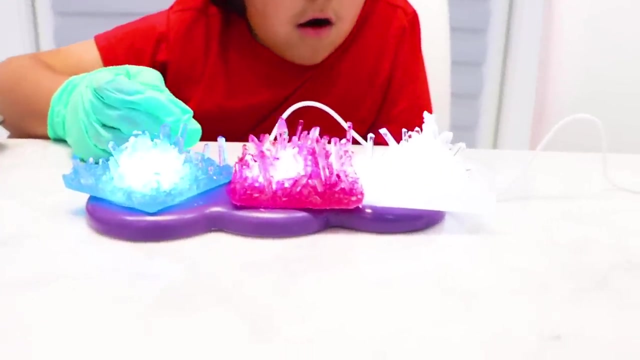 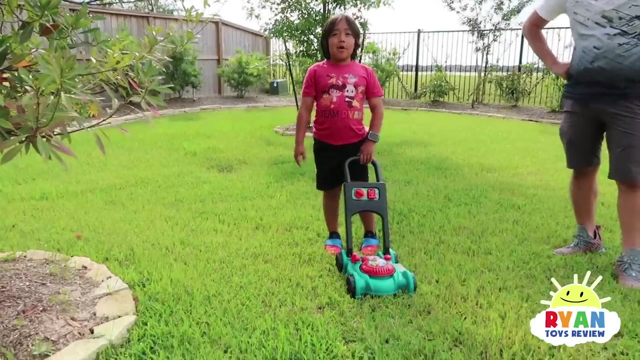 like it comes with a display case and I can put these crystals on the light. she can turn them on like this: oh, that's so cool. good job. it took us about one week to make the crystals. guys, I'm mowing the lawn today. thank you, Raya. 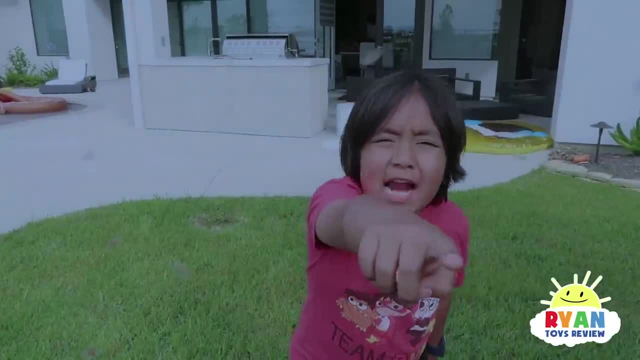 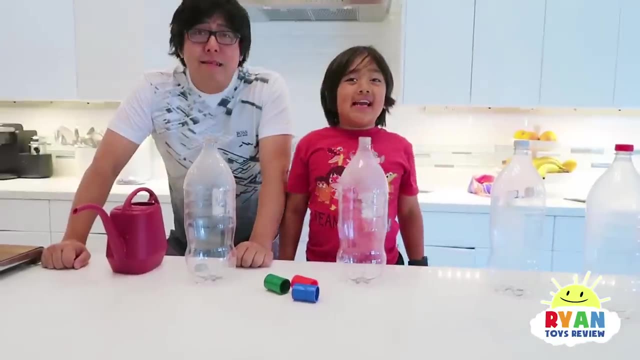 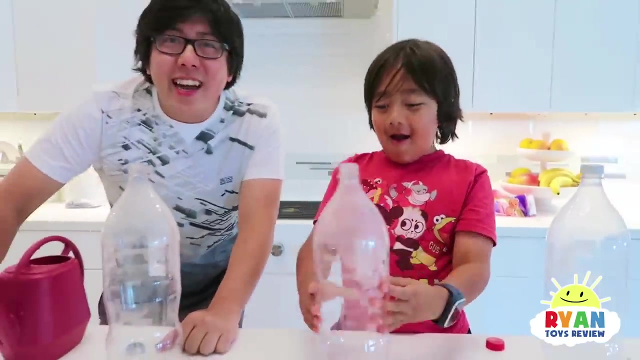 you're a good helper, Daddy. there's a tornado. go back inside the house. I can't believe that was a real tornado, but what if we make our own tornado in a bottle? wow, that's a good idea, Raya. I just really want it all right. good, good job, Raya. I think that's enough. 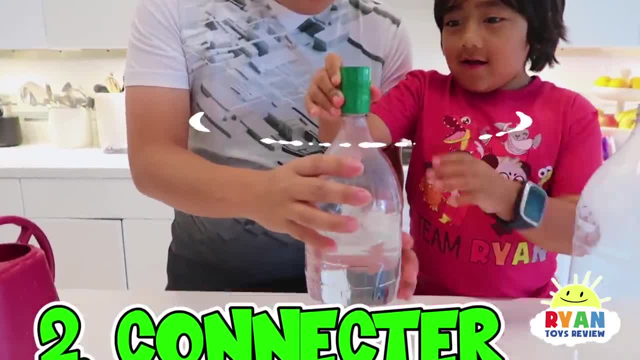 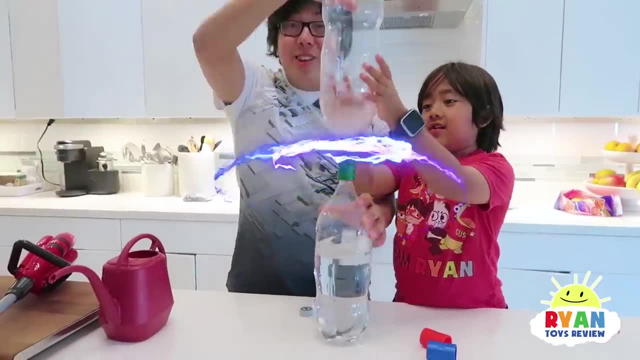 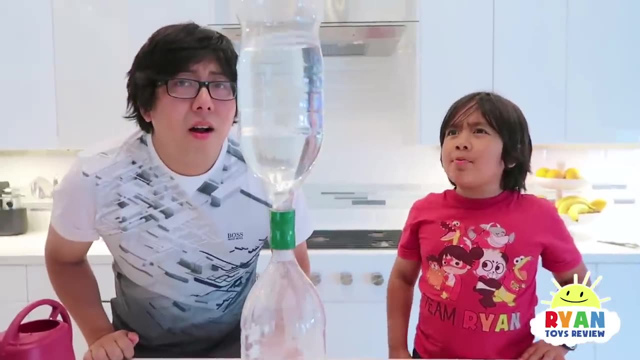 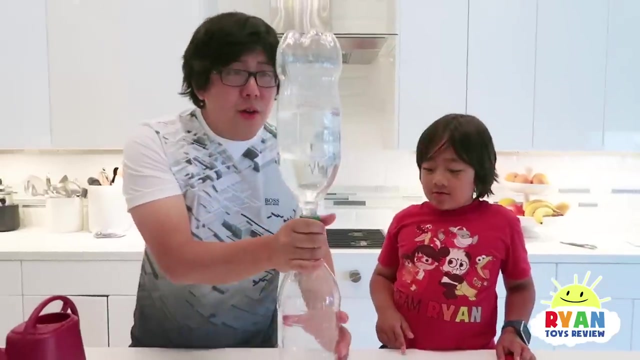 next, I'm gonna put on a connector. all right, okay, twist, twist, twist. good. then this here: wow, it's connected. now, now we do this, there's no tornado Raya, nothing's happening. maybe we twirl it. this part is hard, so I'll do it for you, okay. 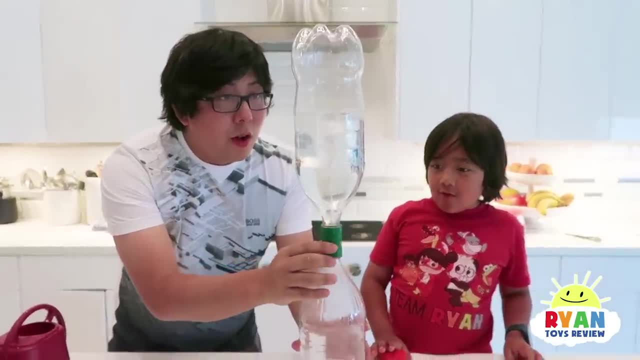 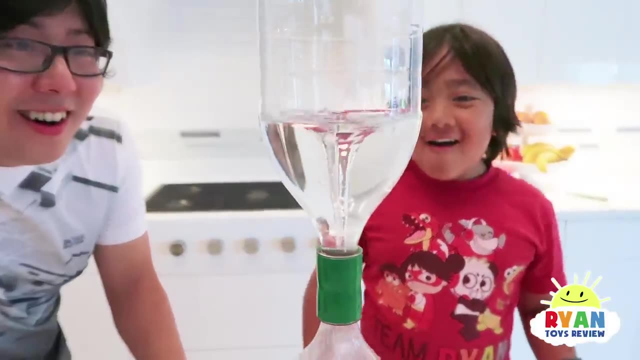 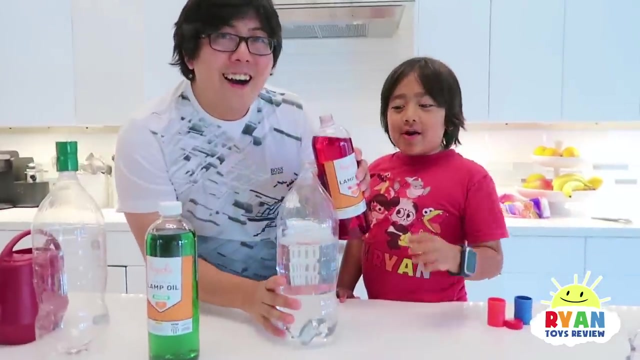 twirl it, twirl it. there you go guys. look, look, look, wow, so cool. look at that, Daddy. what about we add some color? yeah, we can use this lamp oil first. we're gonna try red here. we go, come on in and we're just gonna put it in there. 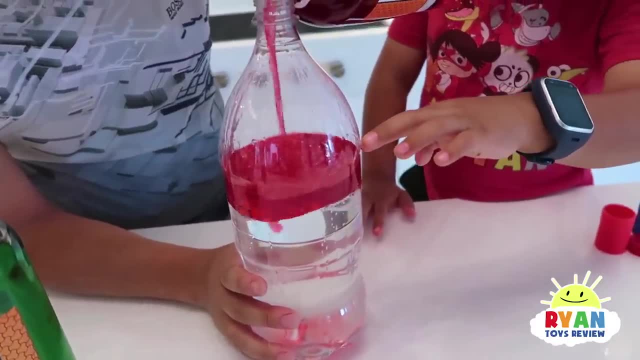 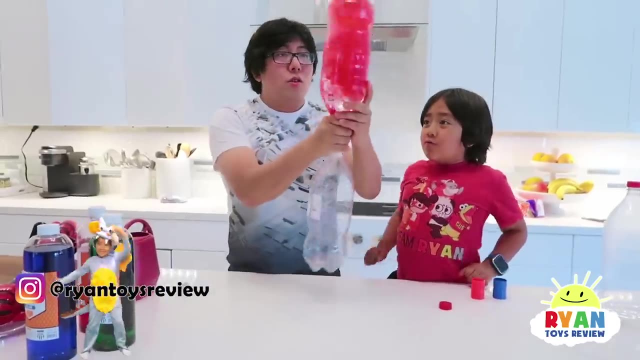 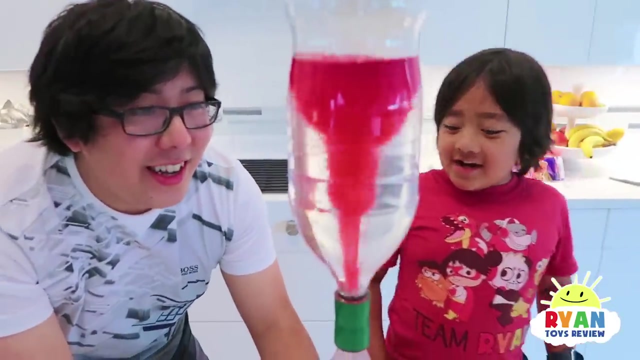 that's good, so good, keep going. yep, almost there done. now connect it again. let's see what happens. are you ready? whoa, twirl, twirl, twirl, whoa. look at that rednado. but you can see the tornado part a lot better. so the center of the tornado is called vortex. 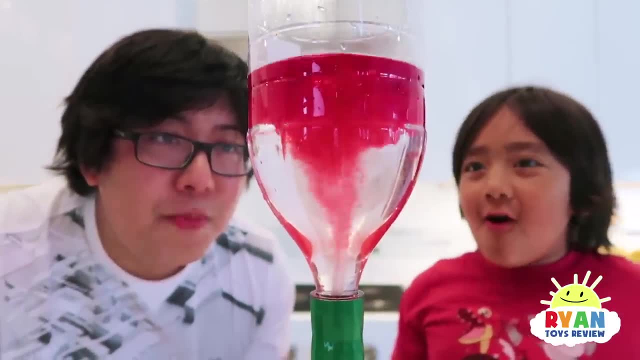 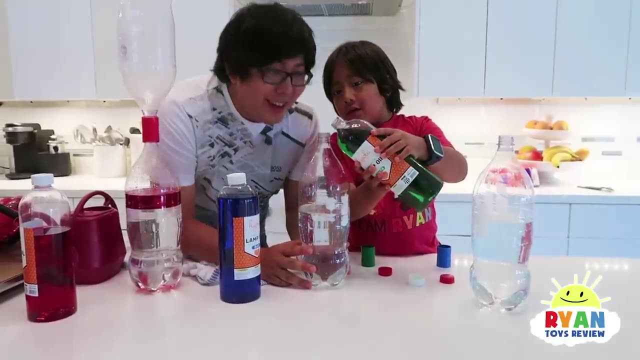 and that's what you see in red. you see that, oh my god, spinning around. now let's make green and blue tornadoes, and I'm ready with tornado 2. oh, we're doing tornado 2. all right, let's start with the green one first. this time Ryan's gonna do it. 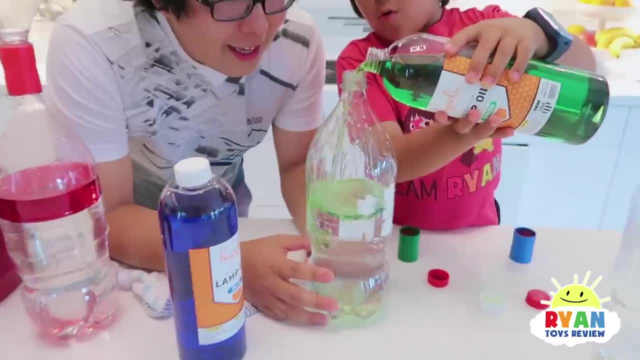 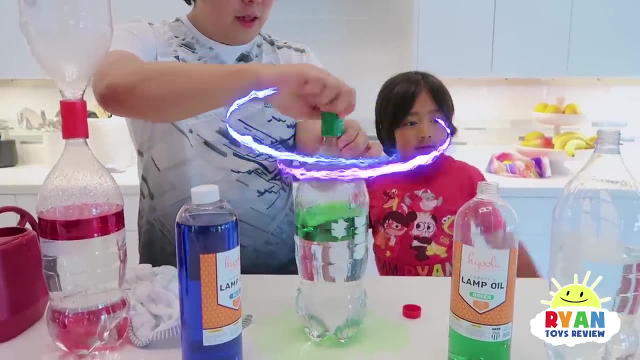 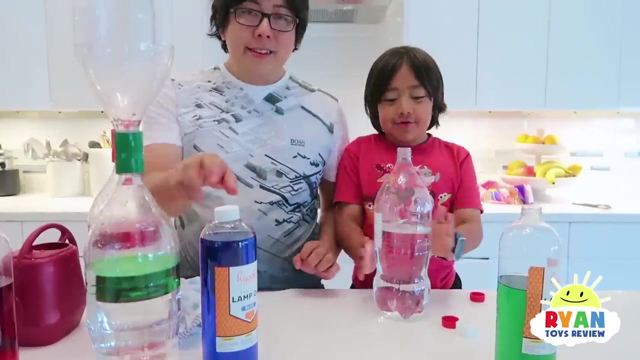 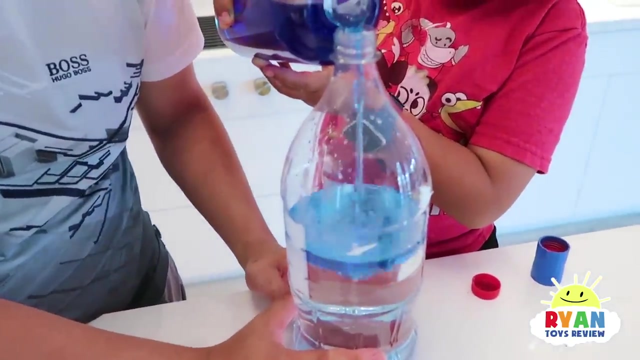 see if you can put the green oil in there. steady, steady, steady. you're spilling it, he's spilling it. all right, good, good, the cap off. give me the yellow one and done. nice, now let's do the blue one. here we go, mmm, steady, steady, steady, steady, steady, steady, steady. 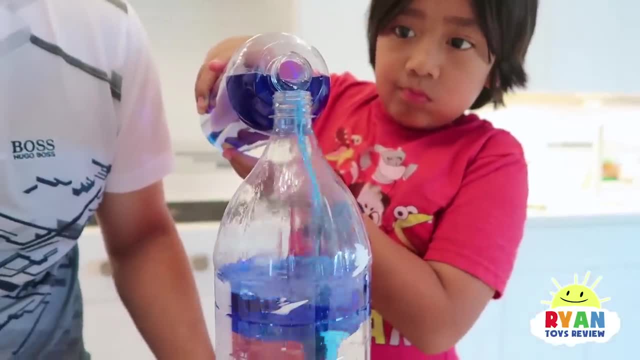 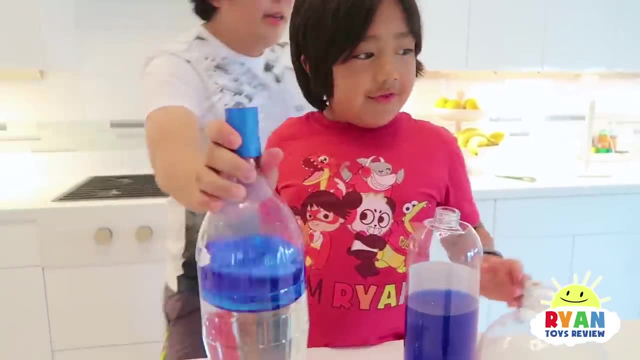 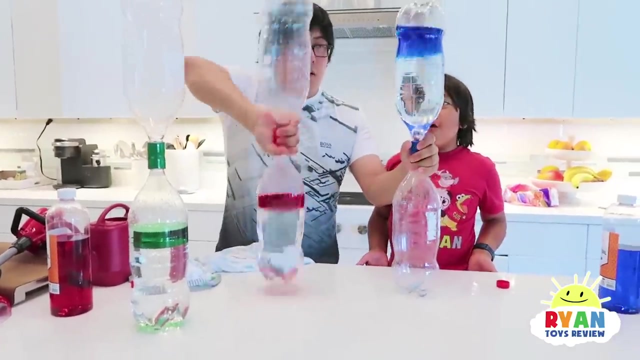 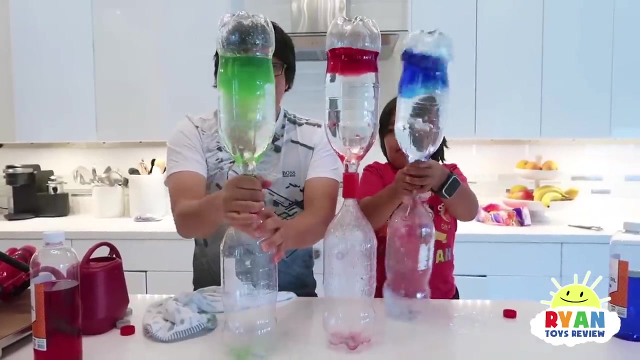 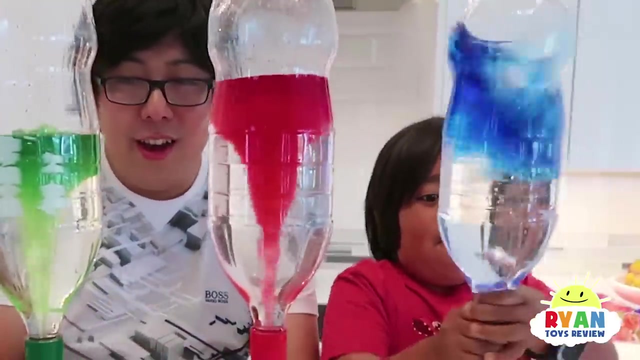 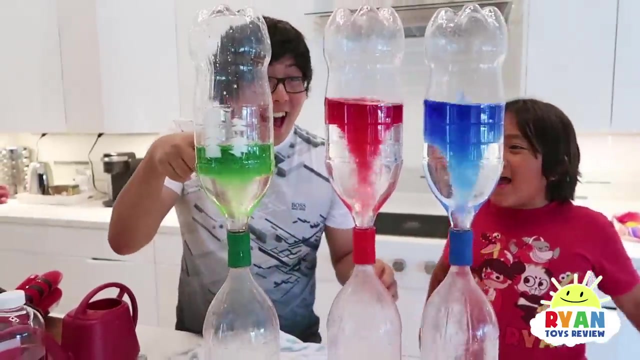 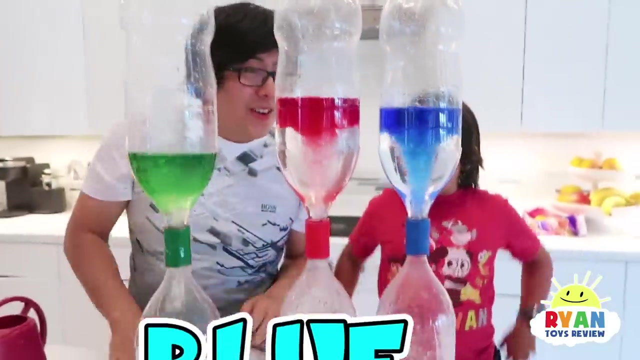 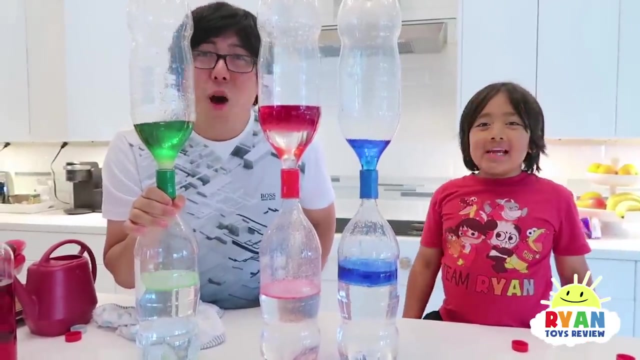 doing good so far going. that's good. all right, good job. let's put the blue cap. there you go. look at that. cool, here we go. cool, nice me, red and blue, so fun. thank you for making tornadoes with me, daddy. nothing you, Ryan. I hope you guys have a fun time and remember, or stay. 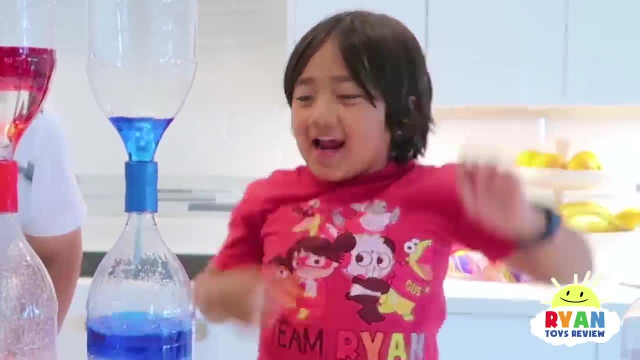 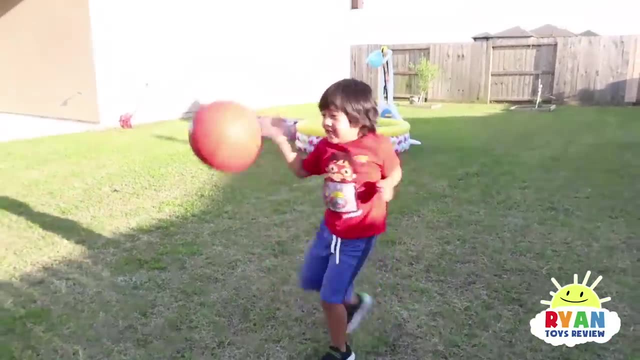 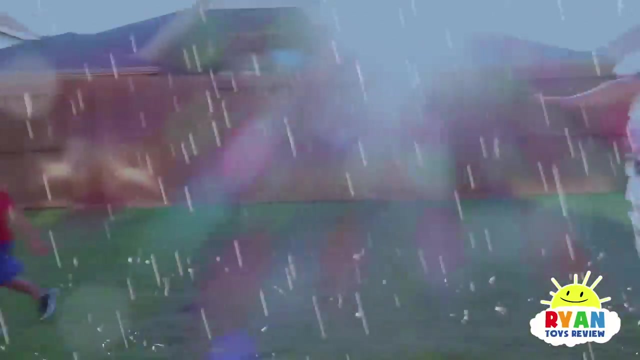 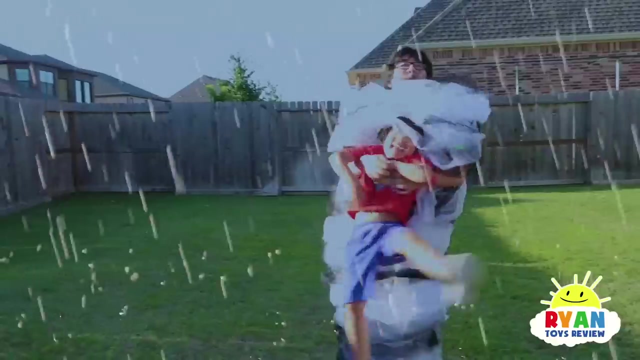 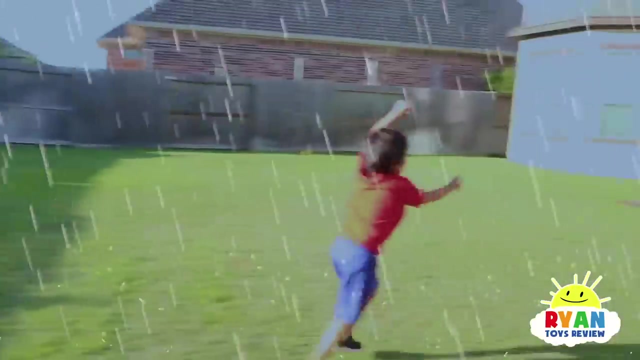 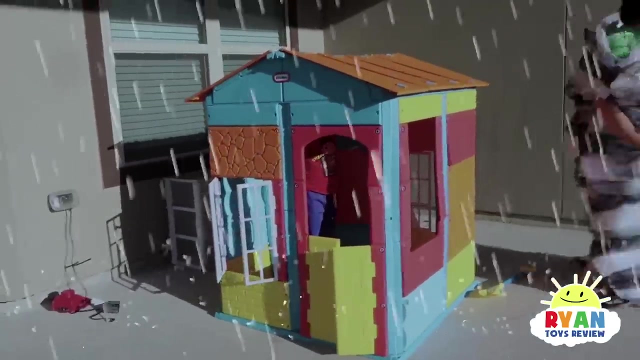 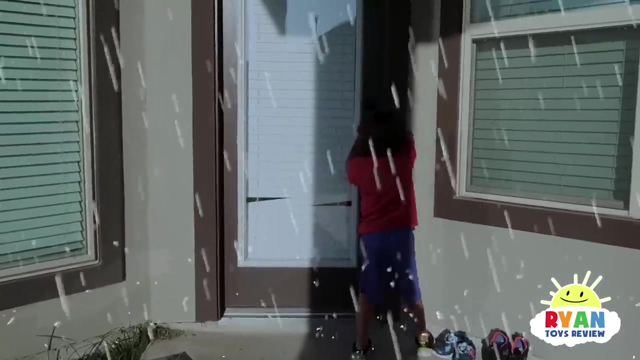 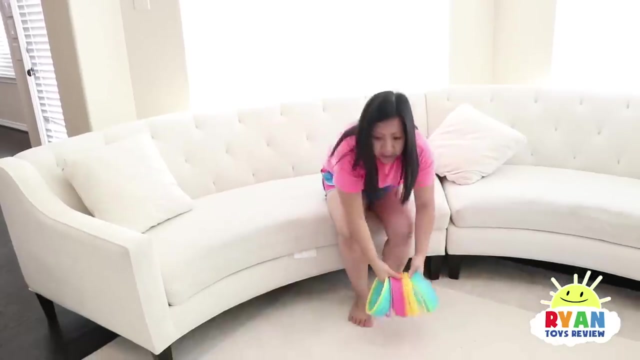 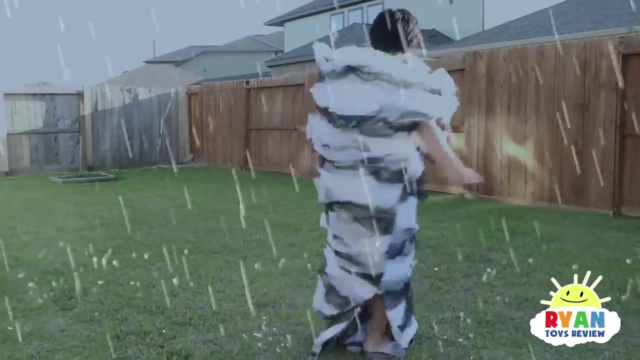 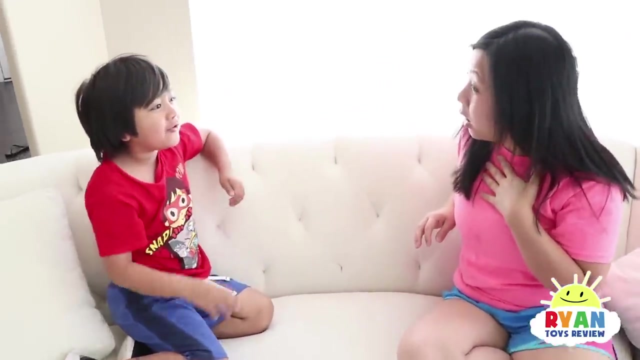 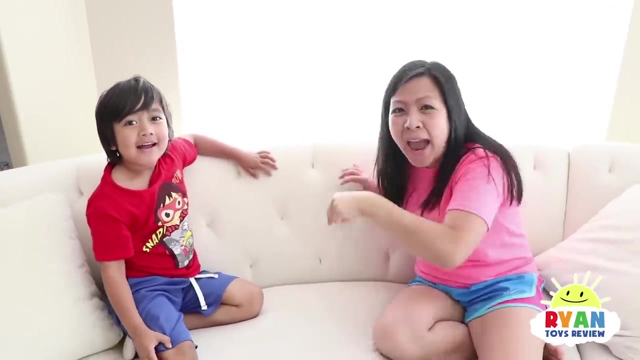 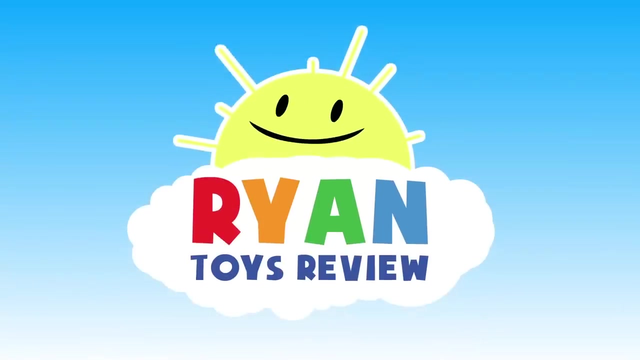 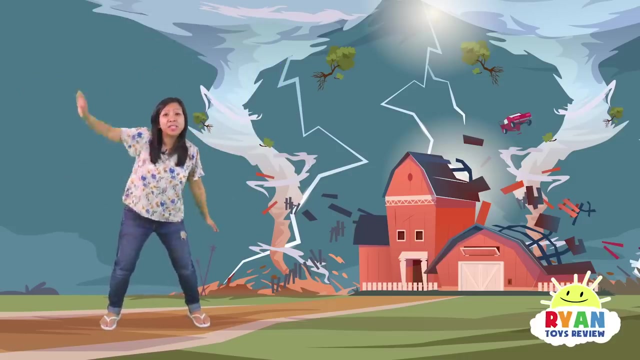 happy and rise up, stay healthy. got you tornado out there? tornado out there. yeah, yeah, yeah, yeah. wow, mommy, how do tornadoes form? good question: how do tornadoes form? I'll be right back. where did mommy go? welcome to Ryan. toy video. hi guys, did you know that our tornado can spin as fast as 300 miles per hour? 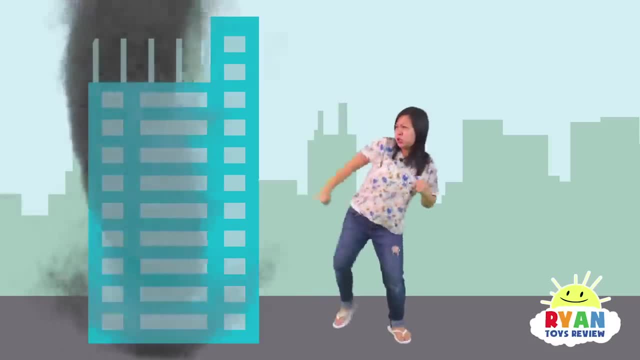 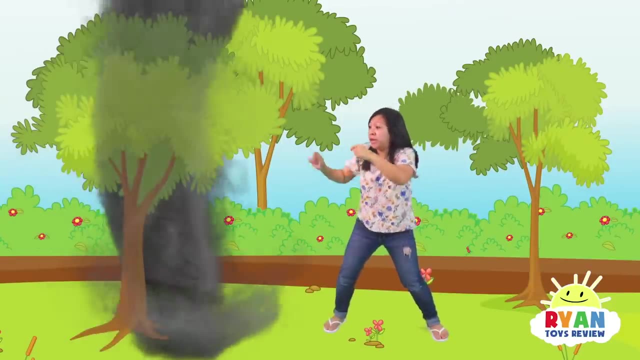 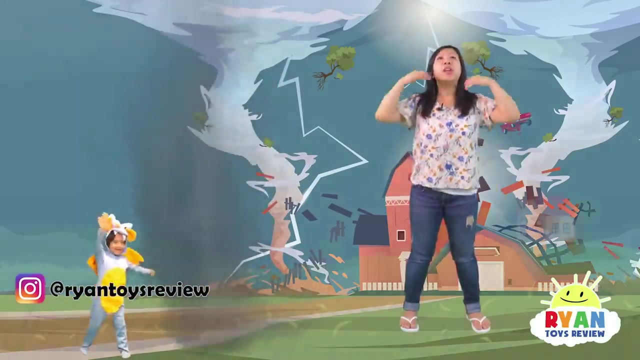 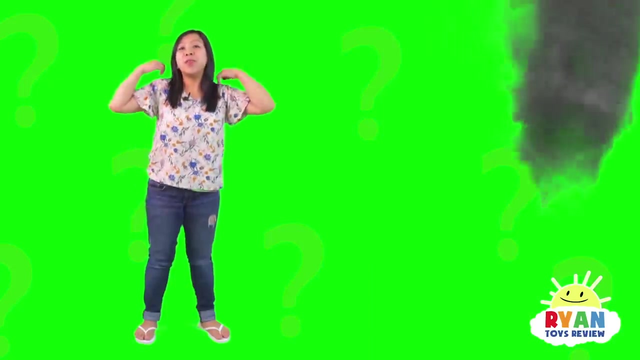 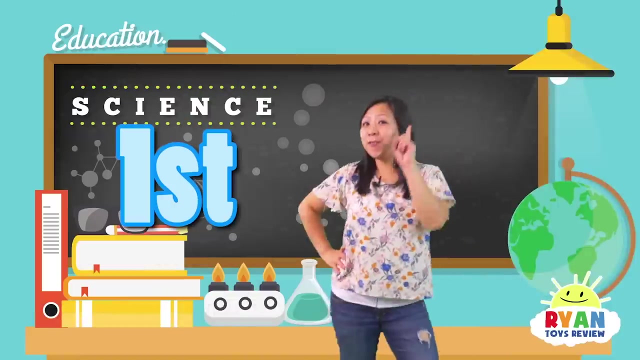 wow. also, our tornado can destroy buildings, power lines- well, look up there- and uproot tree. a tornado is a rapidly rotating columns of air that forms during the storm and connects with the ground through a funnel cloud. so now that we know what our tornado is, we need to know why they form. first, we need a very, very special. 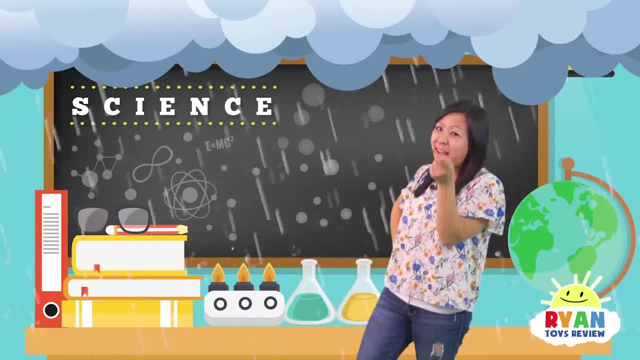 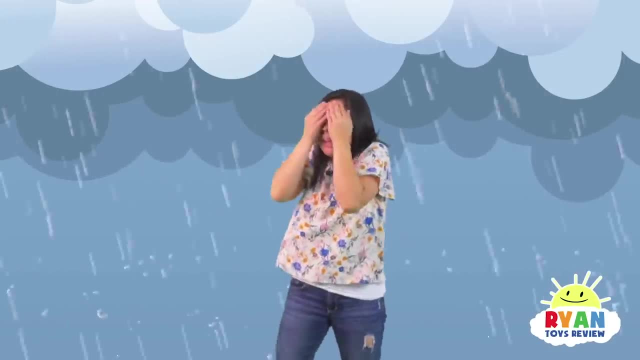 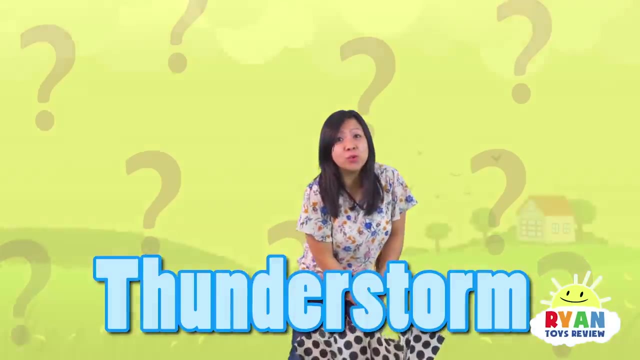 kind of storm? can you guess what kind of storm? it's loud and they can be scary. did you guess what kind of storm? that's right, I'll be right back, but the kind of storm you need to produce a tornado. whoa is caught in a thunderstorm. 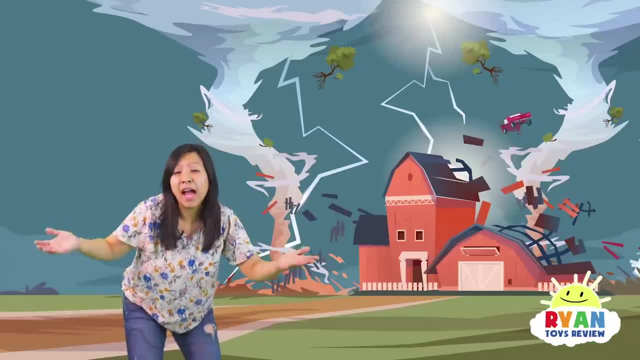 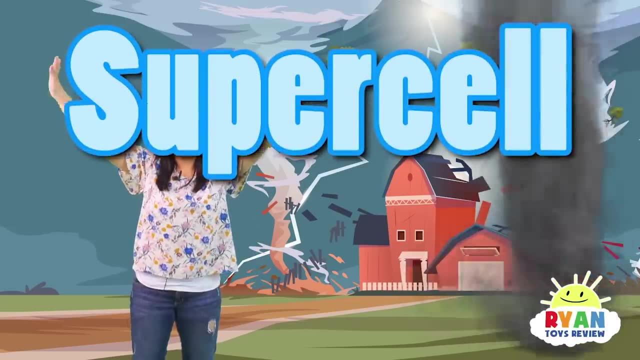 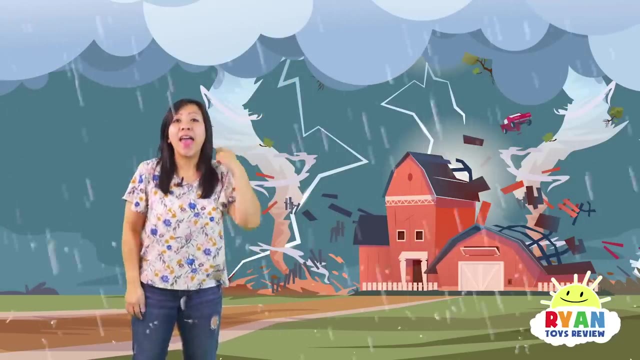 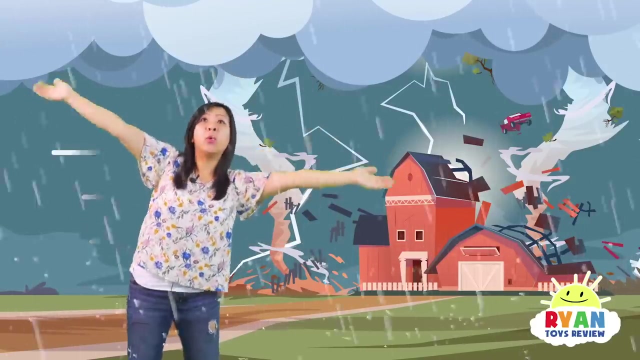 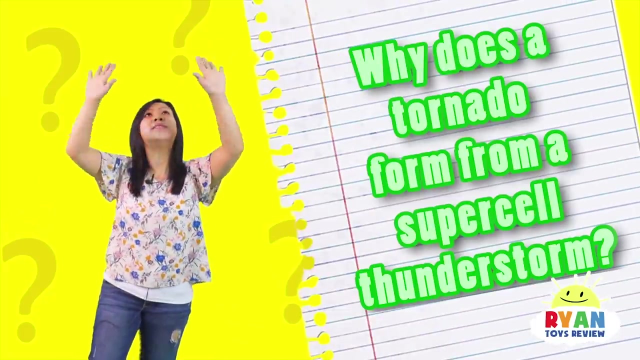 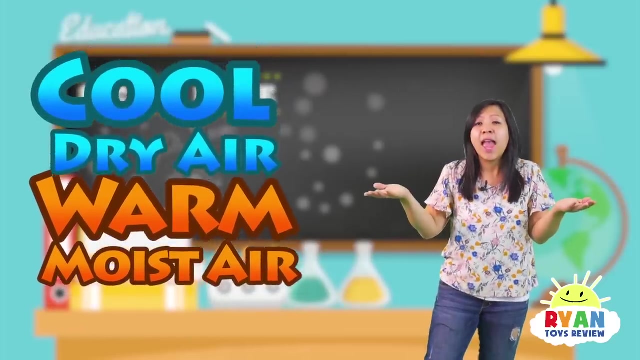 like a tornado. tornado whoa. a supercell thunderstorm. That means it's a storm with rain, hail, lightning and fast wind. Now why does a tornado form from a supercell thunderstorm? It's because warm, moist air meets cool, dry air. 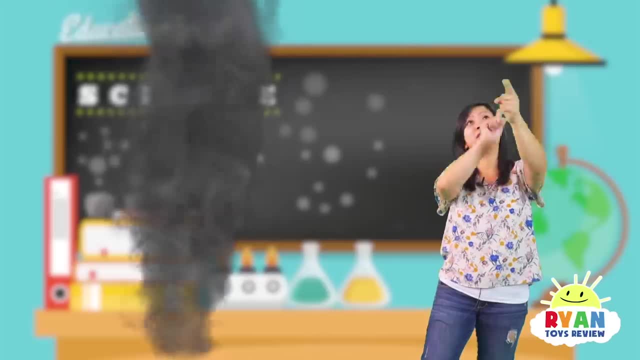 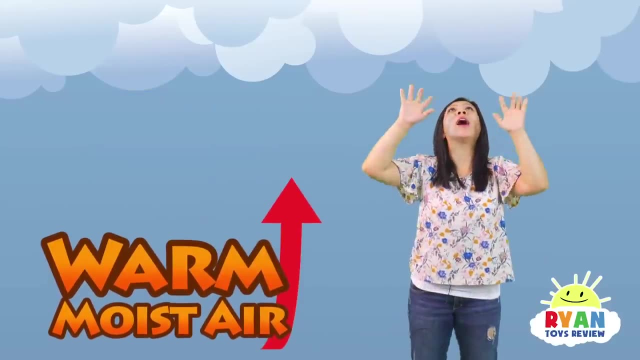 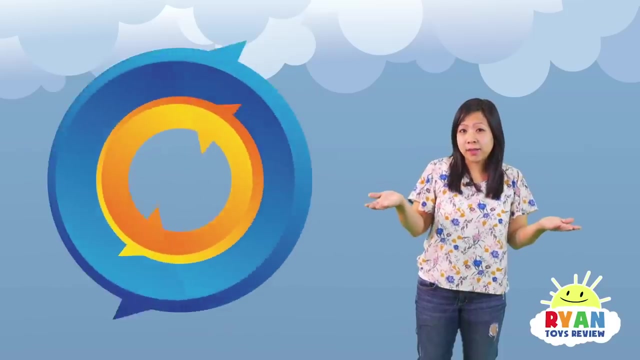 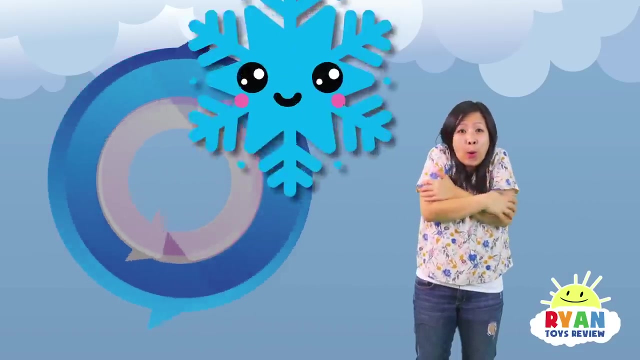 and the wind's direction change. Now let's check it out. First, we have warm air rising. Ooh, cool dry air sinks. It becomes a vortex or funnel where the inside is warm but the outside is cold. It gets stronger and stronger. 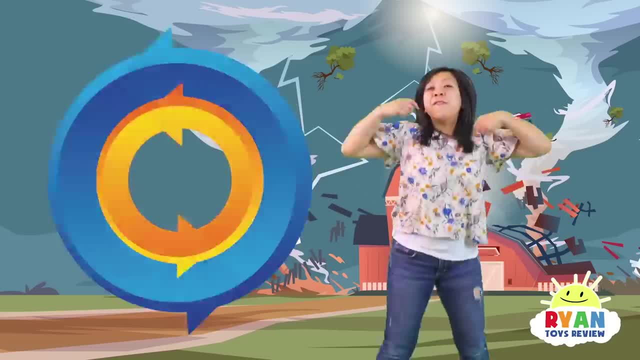 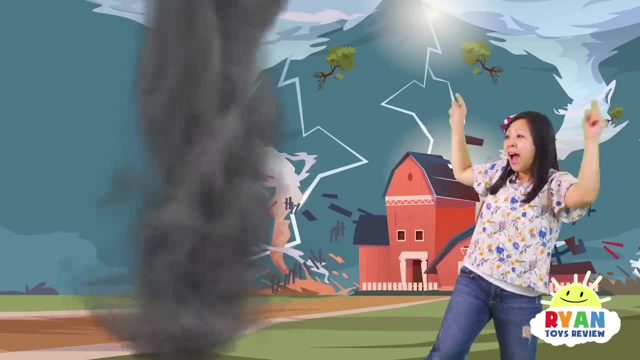 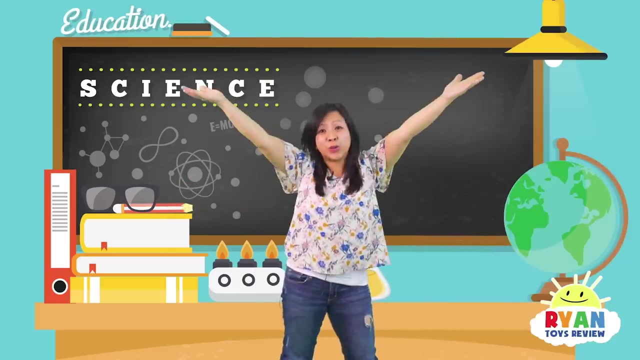 and it spins faster and faster. Finally, it touches the ground and it becomes a tornado. Here it is hi. Now for the fun part. What about we make our own tornado? Are you guys ready to create our own tornado? Look at this. 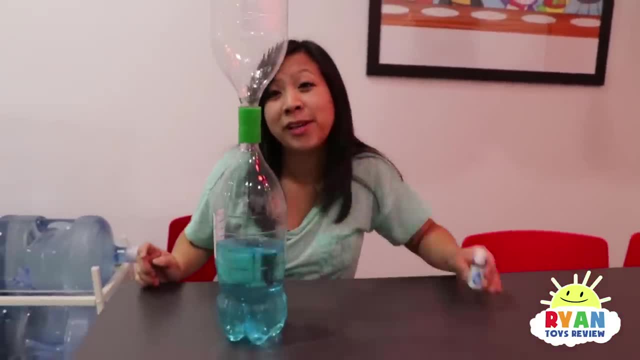 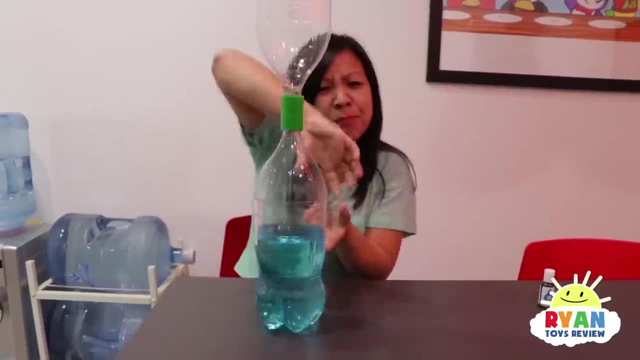 Whoa. so we colored the water blue to make it more interesting. This is heavy. it's like ugh, workout, Okay. Okay, on the count of three, we're gonna flip the bottle over to see if the tornado formed. 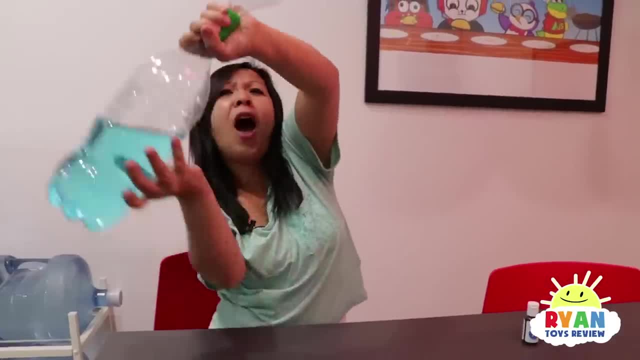 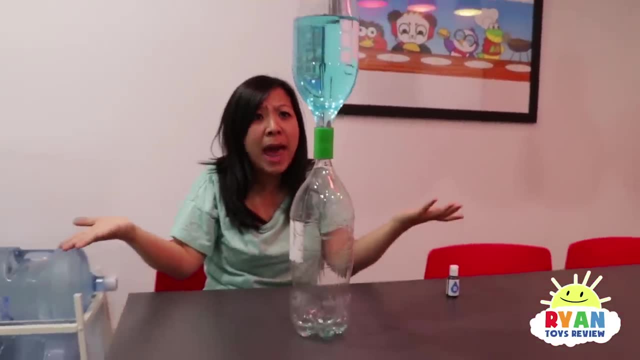 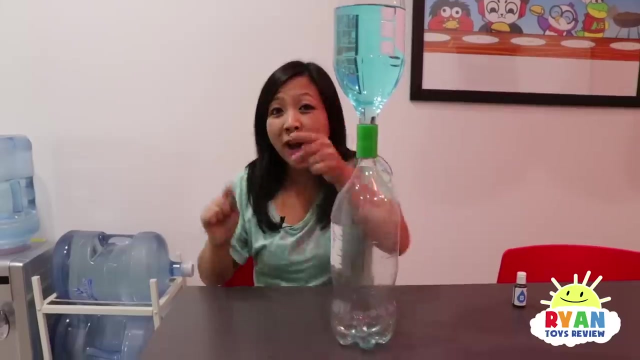 Ready. One, two, three, Yah Bah, Oh no, what do you guys notice? What happened? There's no tornado. Aw, Do you guys know what we should do? What if we try to just swirl the water like so? 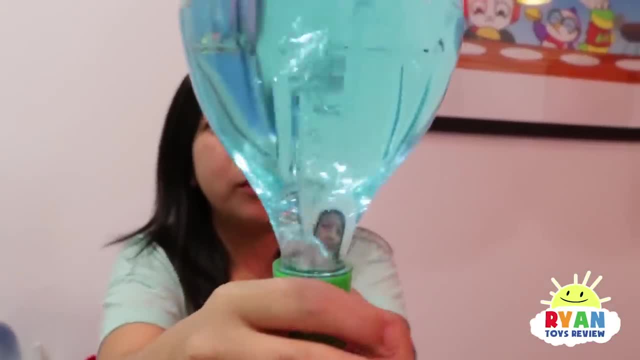 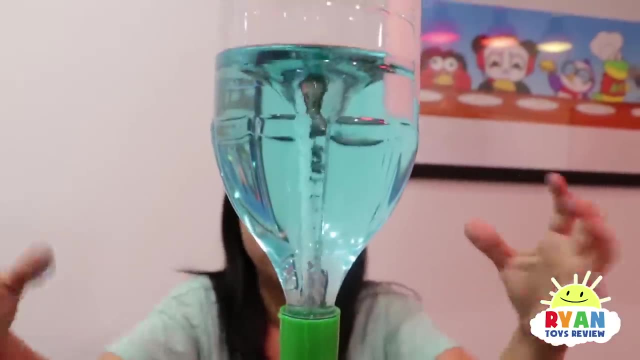 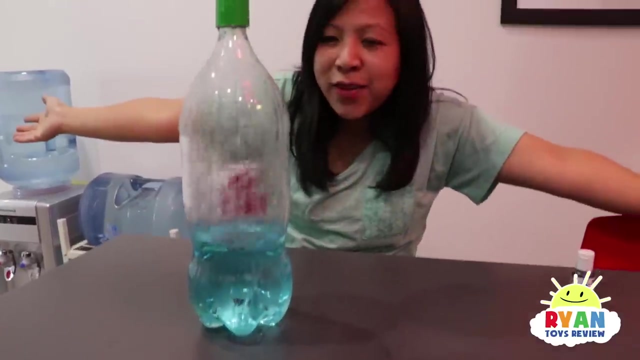 Woo, Oh, oh, oh, oh, Ooh, Whoa. what do you guys see now? Do you see how, as the water begins to move, it creates energy and it makes it flow downwards? Look at that Now. that's a real tornado. 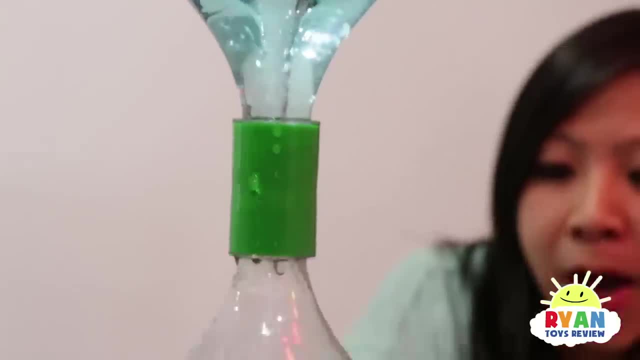 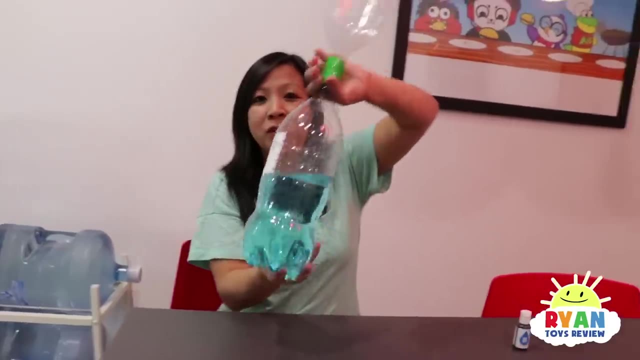 And as the water flows down, the air from the bottom bottle flows up to replace it. That was so much fun. You ready to see it again? Okay, so what do we have to do? We have to shake it, Okay, Whoa, the water's spilling out, but it's okay. 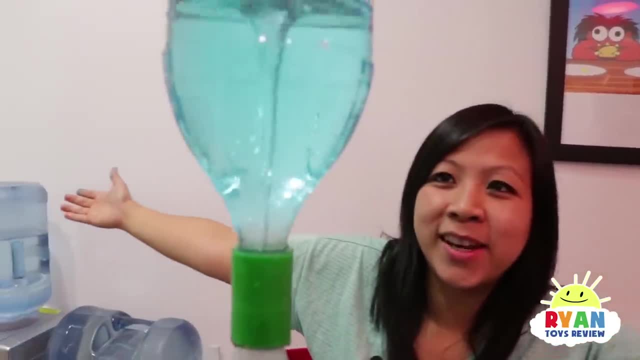 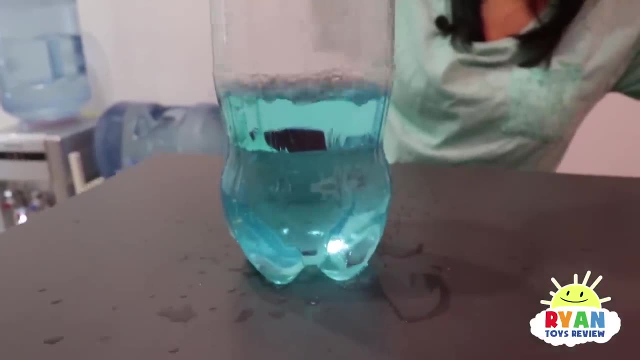 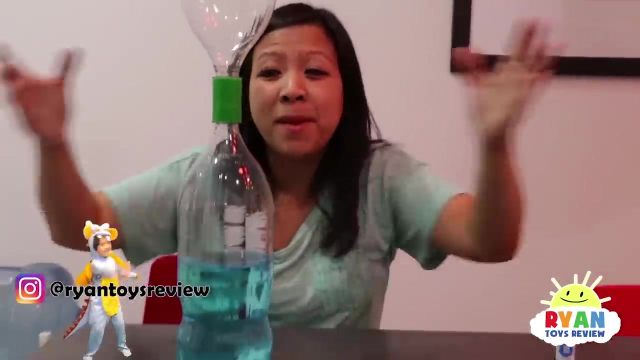 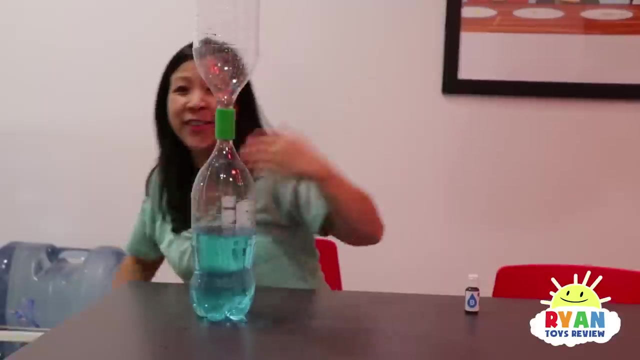 Woo, Whoa. look at that tornado. go, Woo Woo, Wow. that was so much fun making this awesome tornado, But now let's go and meet a real live tornado, Let's go. So now we're at five. 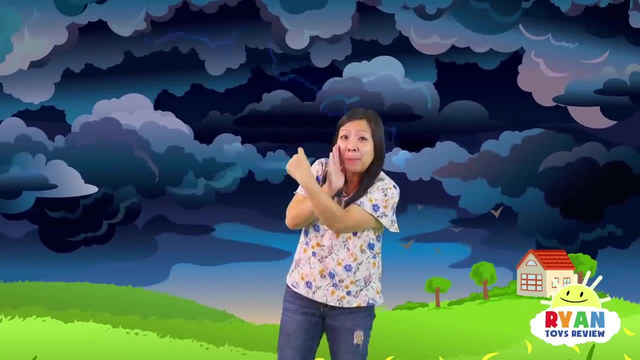 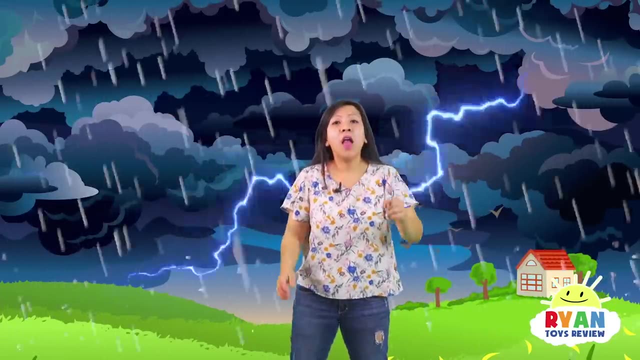 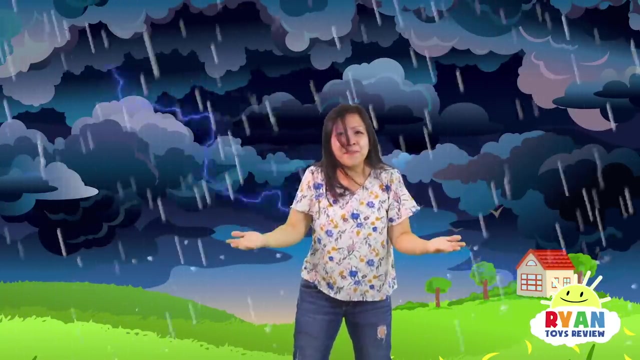 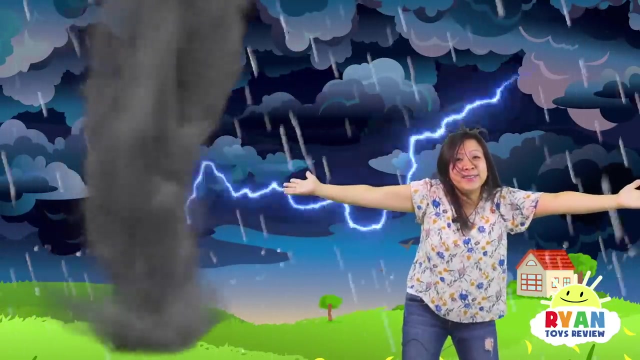 And there's a giant storm happening behind us. Do you guys see it? There's some big clouds here And it's getting. it's getting pretty windy. These are perfect condition for a a- a tornado. I wonder if it's a nice tornado. 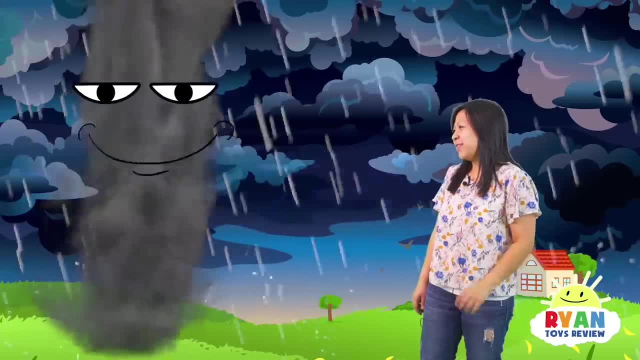 Let's see. Hi man, Hi Mr Tornado. Well, howdy there? Uh wait, What are you doing out here? Don't you know how dangerous tornadoes are? Oh, I'm sorry, I didn't know. 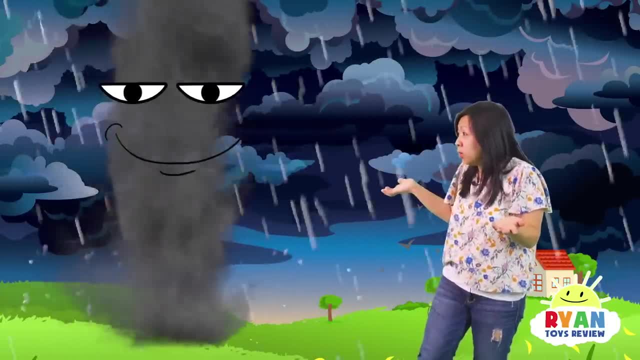 Well, I'll warn you a little bit about us, But you have to promise to keep yourself safe if you ever see one of us again. All right, Okay. So what makes tornadoes so dangerous? Well, you see, we spin really fast. 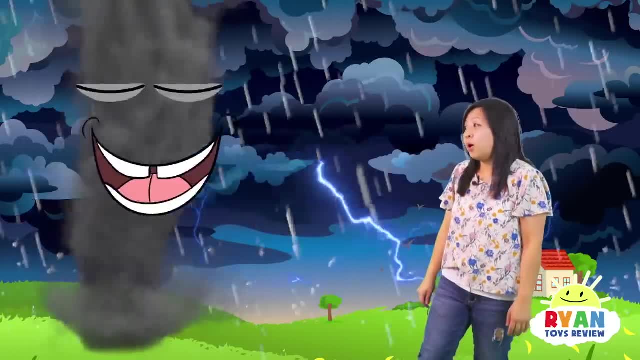 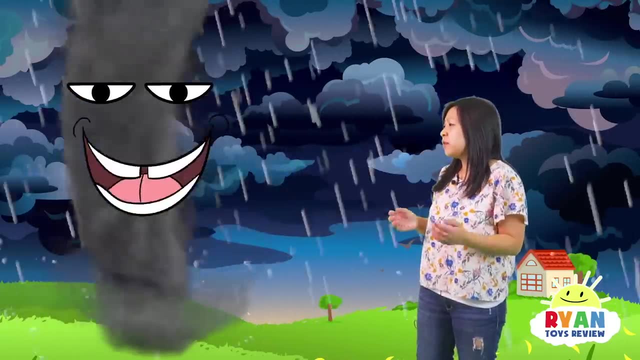 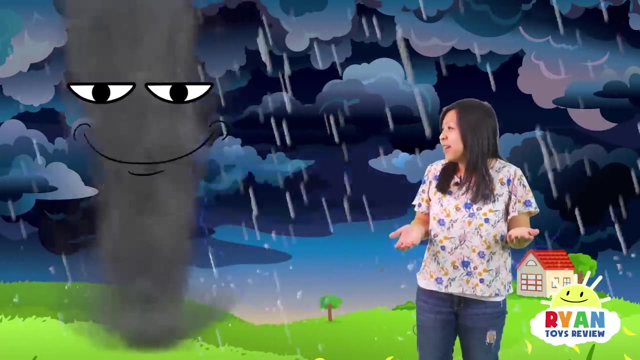 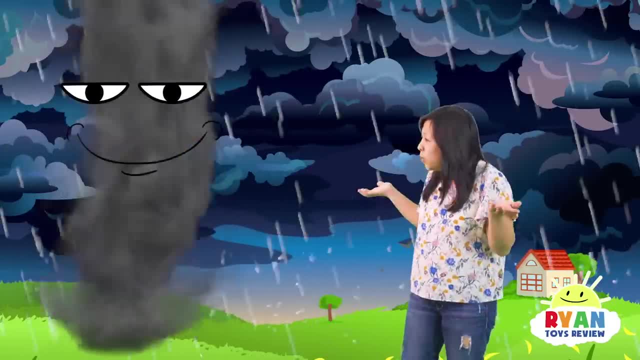 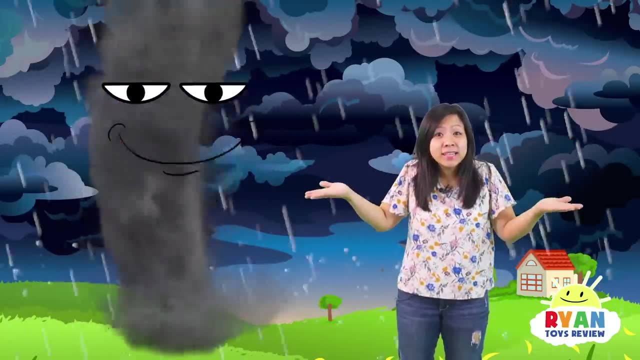 Some of us can spin that fast. We're also unpredictable too. So what does that mean? That means we can pop out of the storm at any time, at any place, and it can be a weak tornado or a strong one. You don't know till you know. 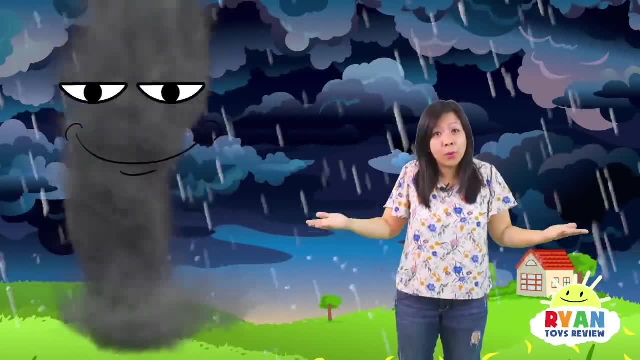 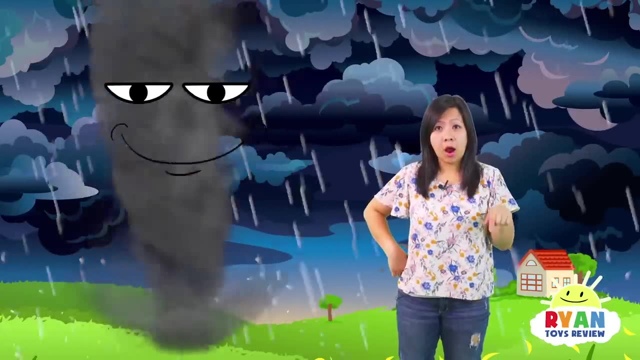 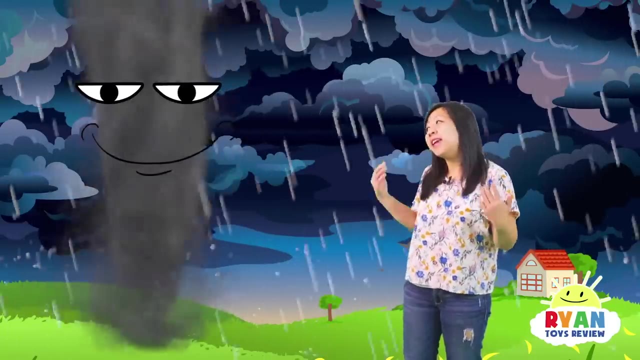 You know. So what are we supposed to do? If you have a basement, get to it. If you don't, go to the lowest floor and find a safe place in your house that isn't close to windows, like a bathroom or a closet. that's some good advice. thank you, that's right. so get on and get. 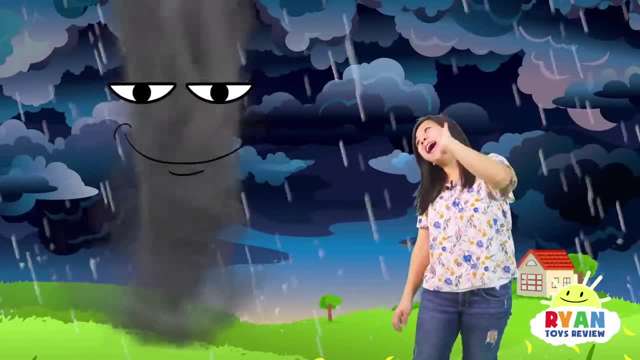 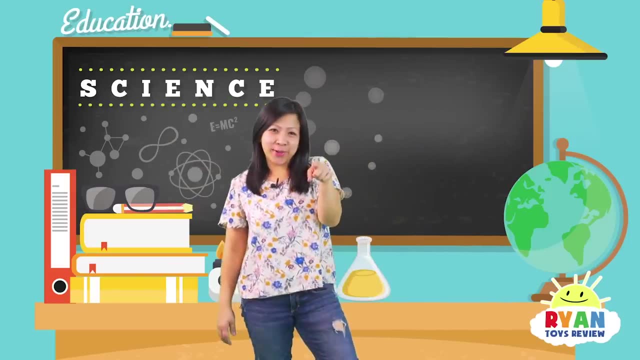 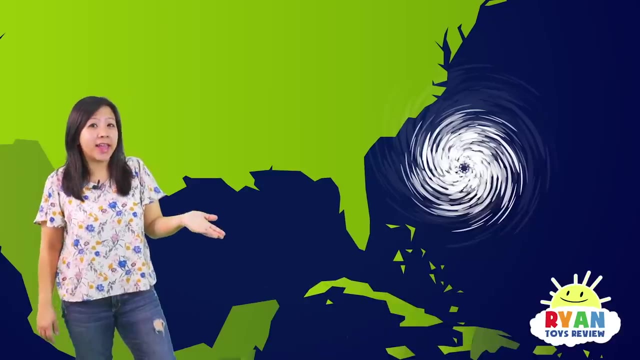 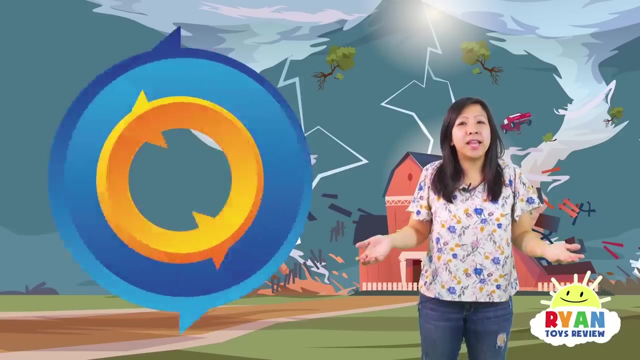 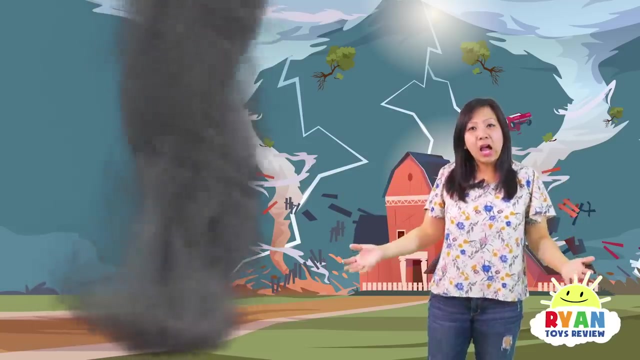 safe. okay, thank you so much, mr tornado. bye. so now that we know so much about tornado, let's take a quiz. question number one: what is a tornado? is it a hurricane? is it your best friend, or is it rapidly rotating columns of air that connects a thunderstorm to the ground? that's right, a tornado. 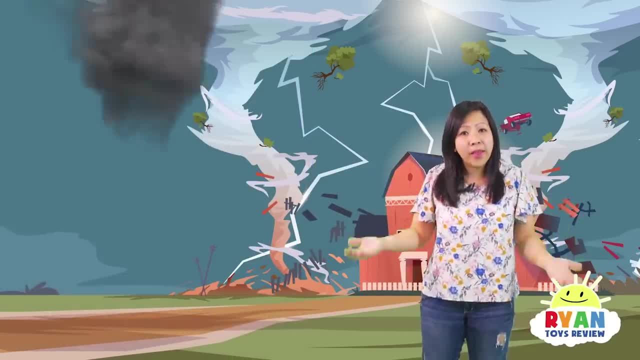 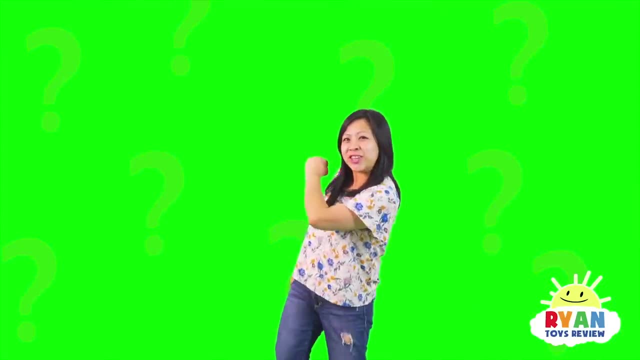 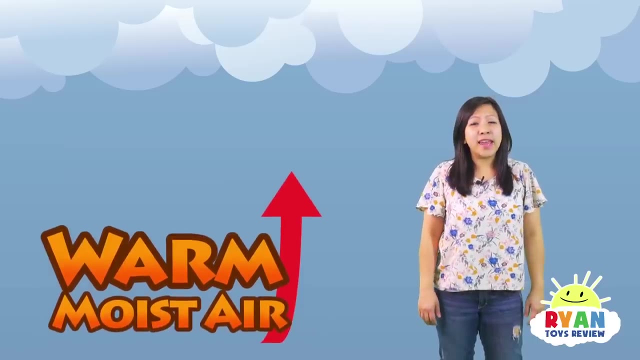 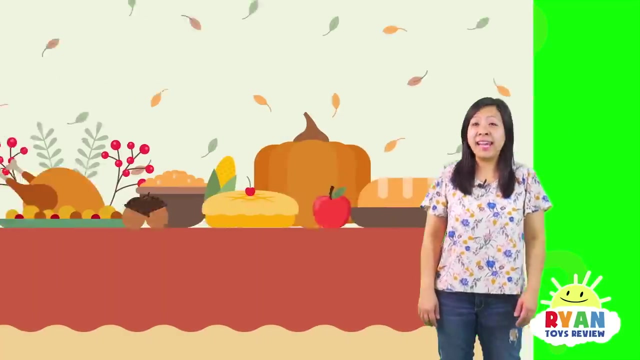 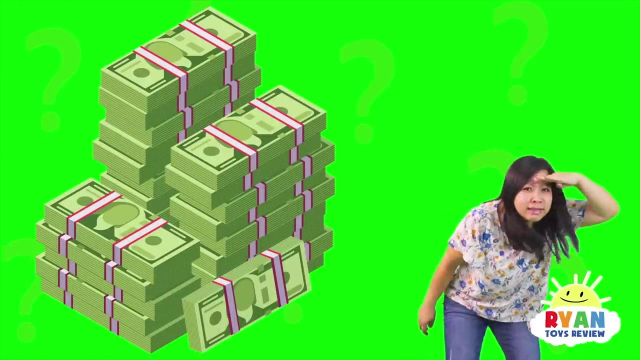 is a rapidly rotating column of air that connects a thunderstorm to the ground. next question: why do tornadoes form? is it because warm, moist air meets cool, dry air and wind direction changes? is it because they are late for dinner? or is it because they are looking for their money? that's right. a tornado forms because when they go up to the surface, they're eliminated, and that's why they stretched out. she solved this. one, two, three, four, five, six, seven, eight, ten. I'll show you what happens when tornado forms. the images that are shown on our screen are aprender10 to practice in zooms. to ya spin up Extremadura. 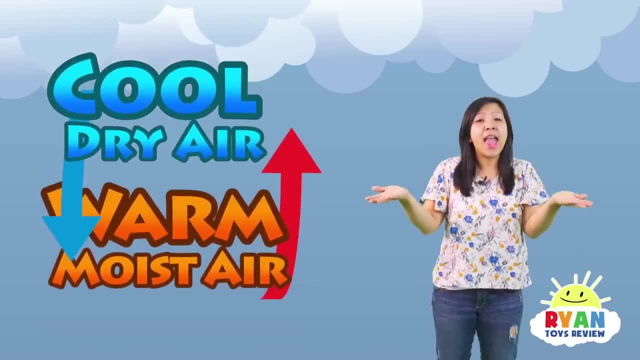 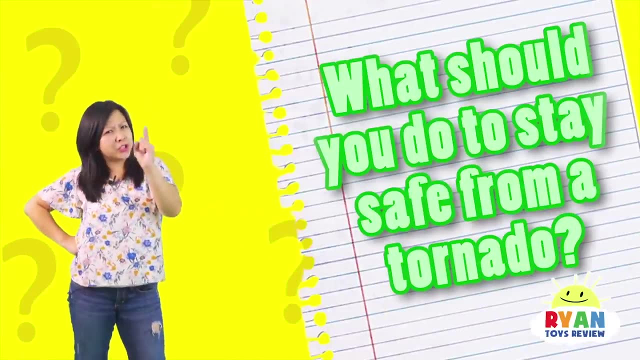 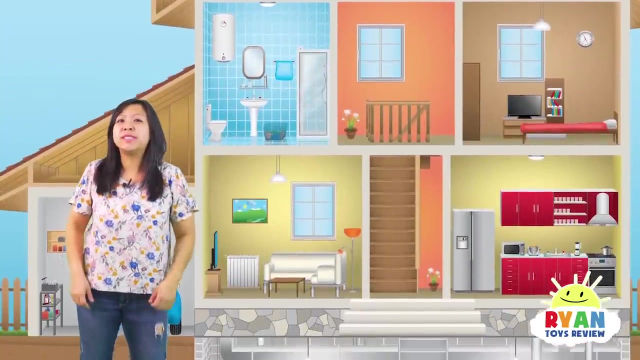 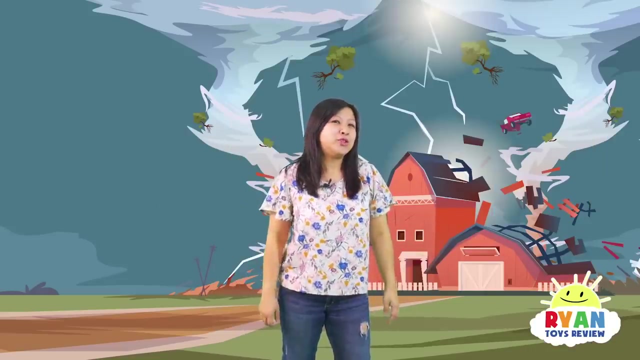 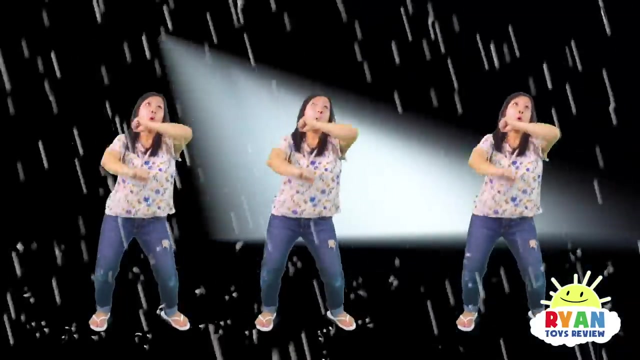 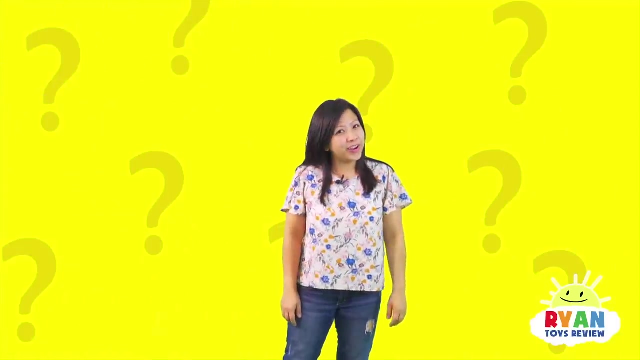 warm, moist air meets cool, dry air and the wind direction changes. question three: what should you do to stay safe from a tornado? is it let's go to the basement or safe room on the lowest level with no windows? or should we dance in the rain? or, if there's a tornado, should you just eat some yummy candy and watch youtube videos? 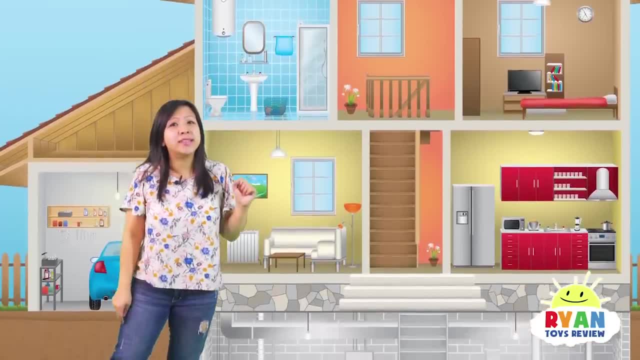 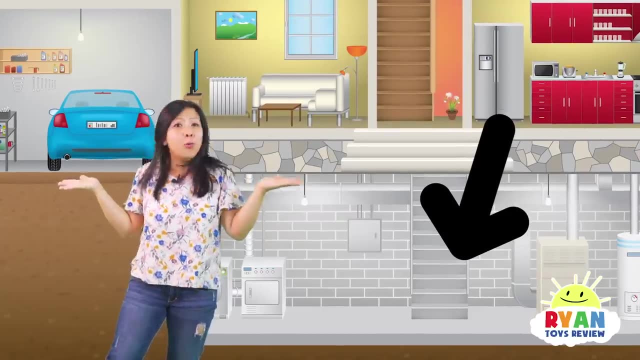 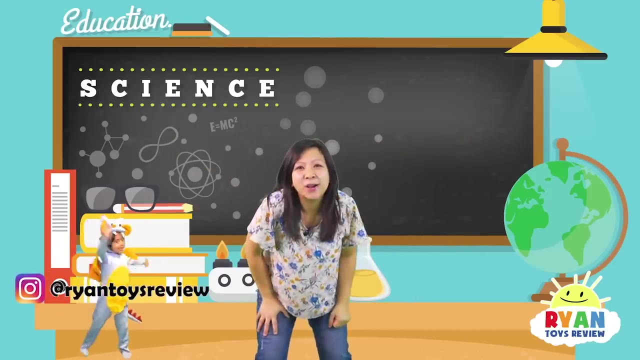 that's right. if you see your tornado, the best way to stay safe is to go to the basement or a safe room on the lowest level where there is no window. great job, now that we learned so much about tornado, let's go back and tell ryan: okay, let's go. whoa, that's how our tornado is formed. 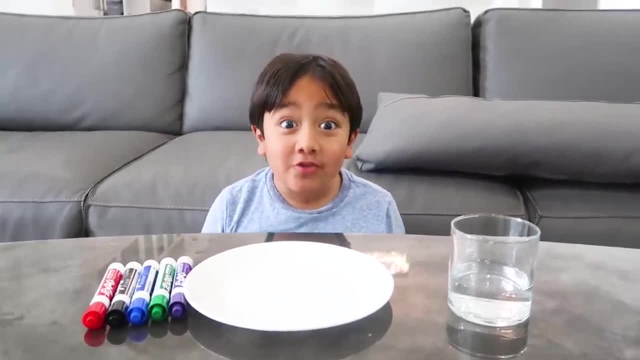 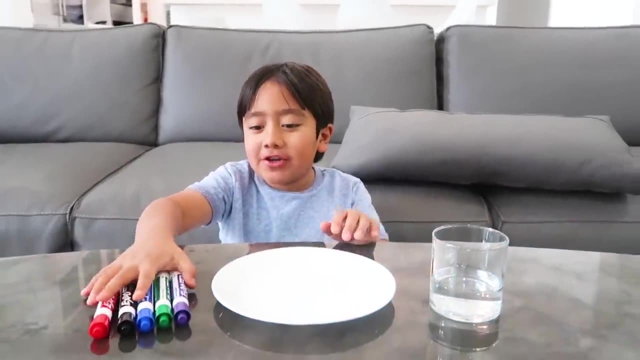 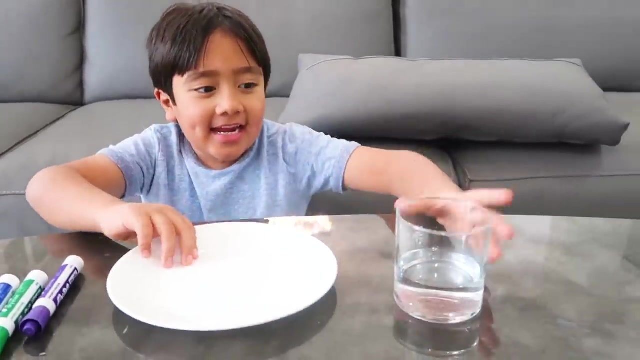 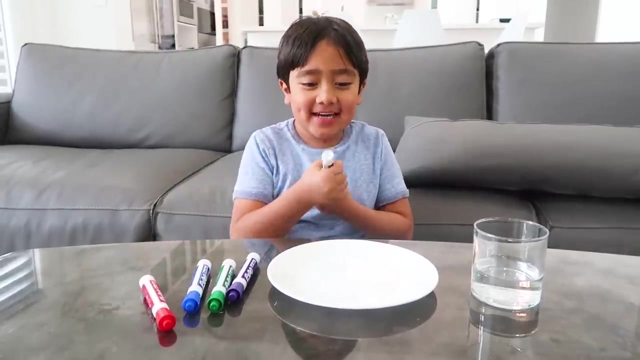 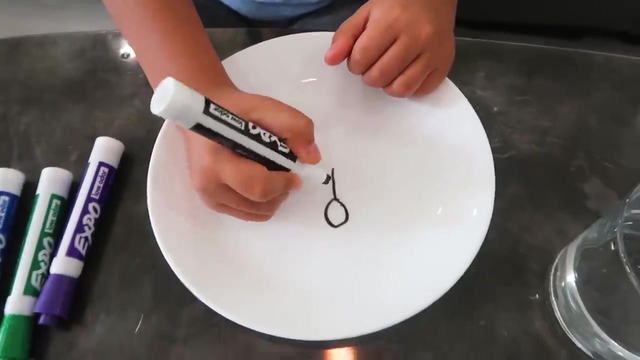 hi guys, today we're gonna put our trawling and then make it float on water. so this is very easy. all you need are some markers, a plate and some warm water. first, draw what you want on the plate. well, i'm gonna make a stick figure with multiple arms plus. so, like this, make it really thick. like this. 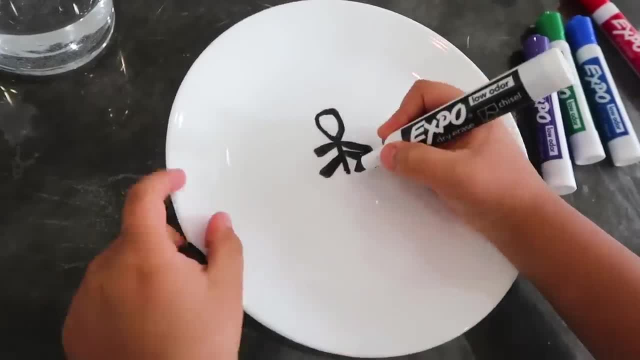 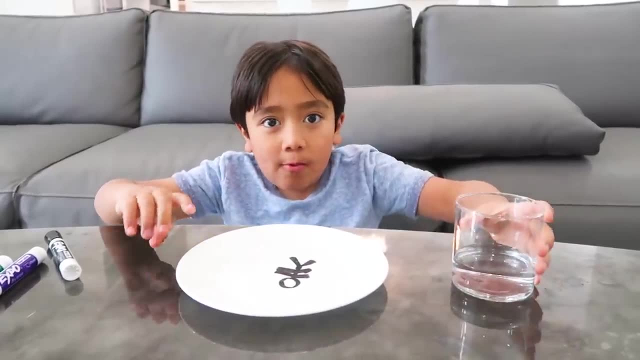 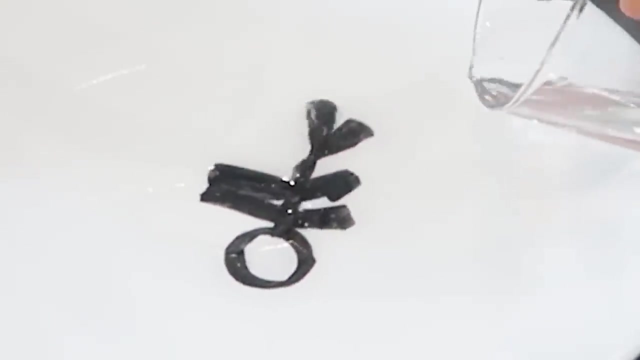 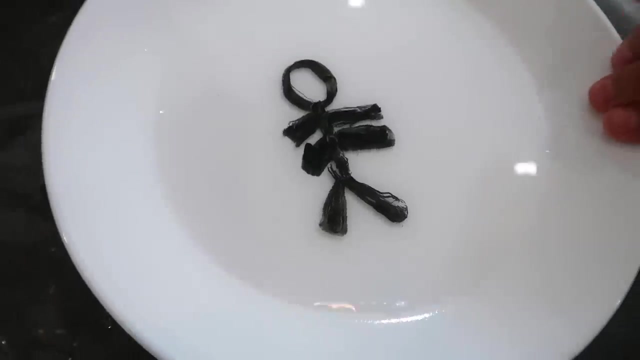 and you make arms and then you make the legs. so after you make your drawing, then you put some warm water on the side. oh, he moved, look he's dancing. oh, his arms too. oh, i feel like the arms or legs gonna break. oh, it's moving now yay. 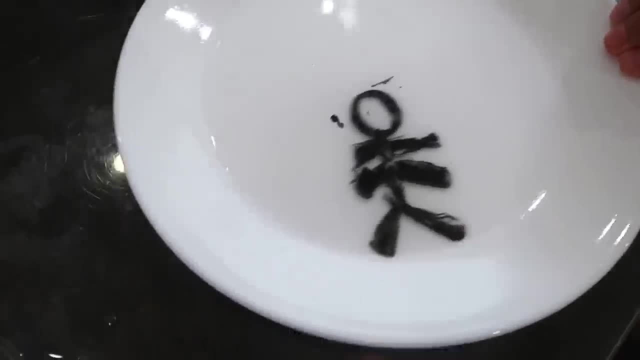 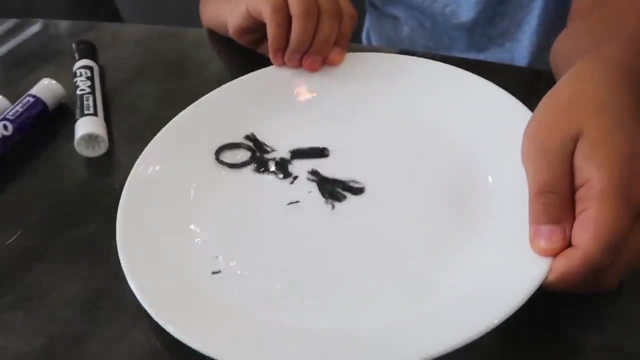 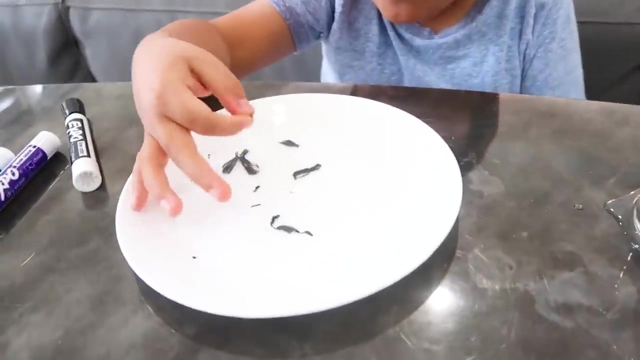 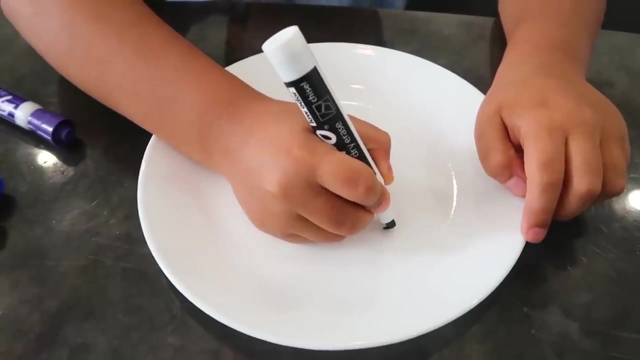 now he can just walk there you go. this is easy way to make your stick figure float. he broke. this is so cool, you can hold it. okay, guys, for the next one i'm gonna make a dog. it should be like this, and then maybe i can put like ears. 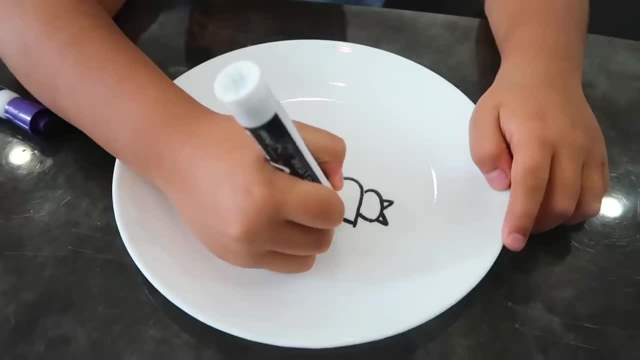 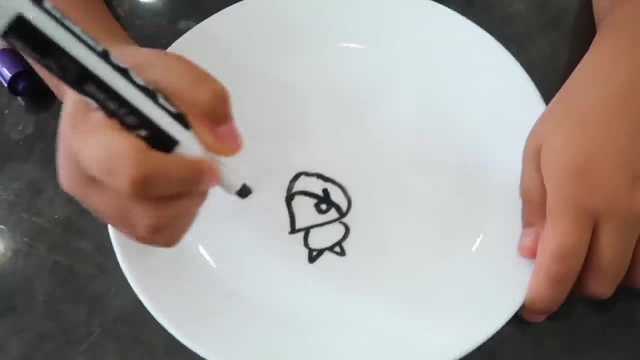 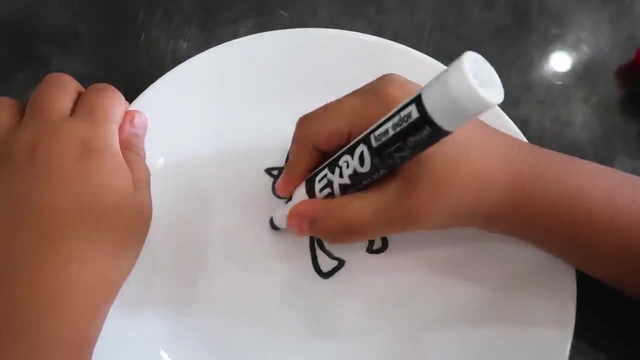 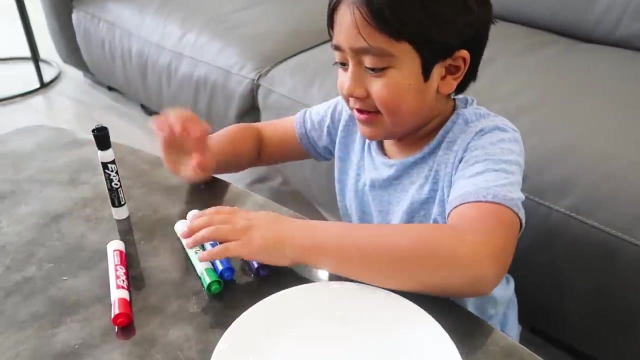 i feel like i'm making a cat. i'm making a big dog or cat. oh, i can't do it right unless i do like this. i put an r, okay, then i'll make the legs and then the arms. i feel like i'm making like a super strong cat or something. okay, now i'm going to put.